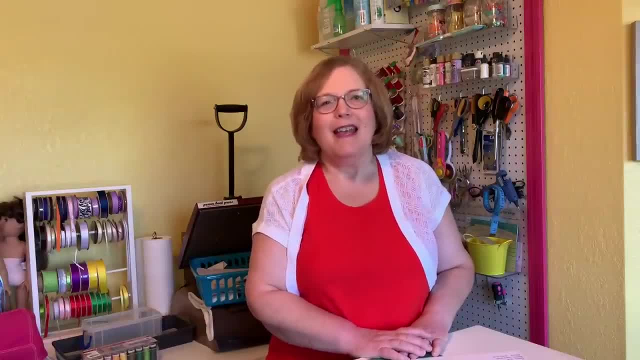 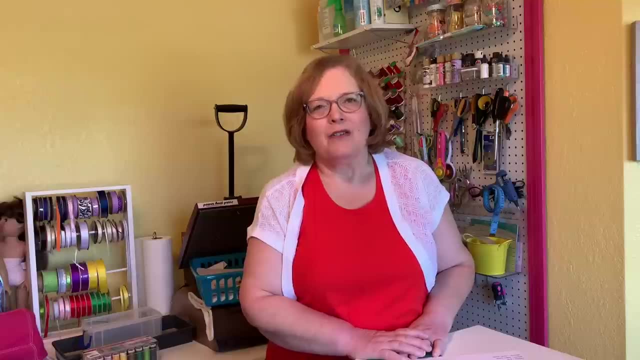 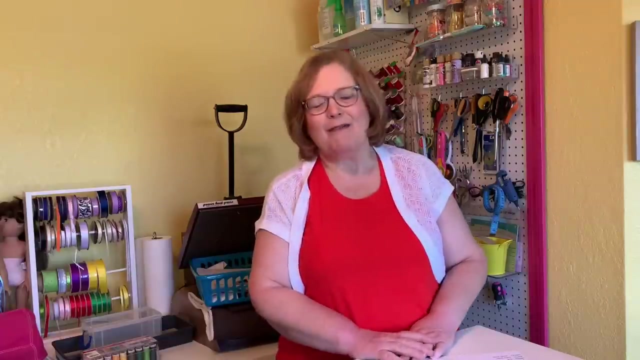 granddaughter will be 13 in January, and it has been a wonderful bonding experience for us, and it has also been a lot of fun, and they have loved, I think, pretty much everything I've sewn for them. Let me just start off, though, by inviting you to subscribe to this channel, if you haven't already. 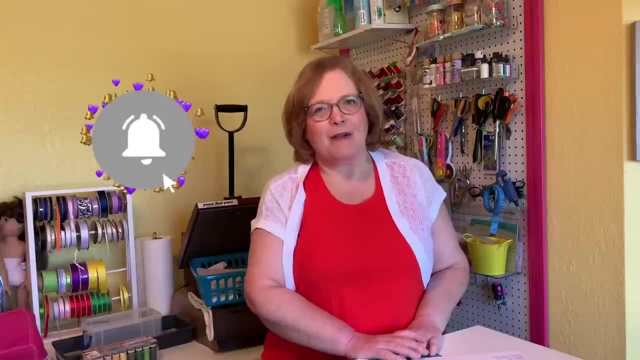 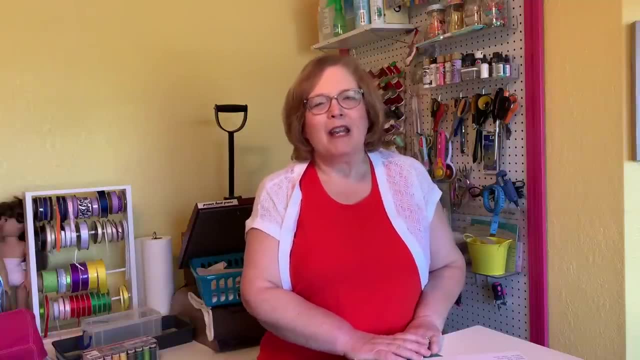 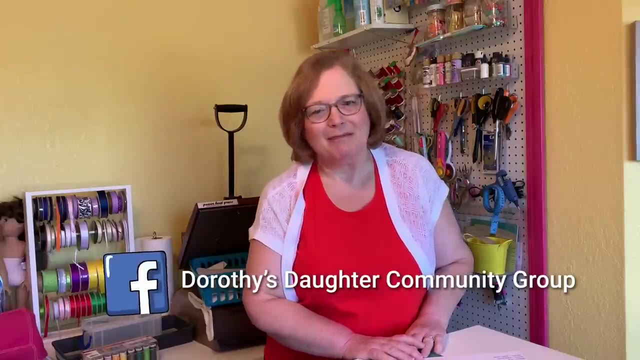 We have a growing community of sewists who help each other out. We have regular chats. We have a Facebook group that we communicate in. I also produce one to two videos per week to keep us all growing in the right direction with our sewing. So what I'd like to do today is share. 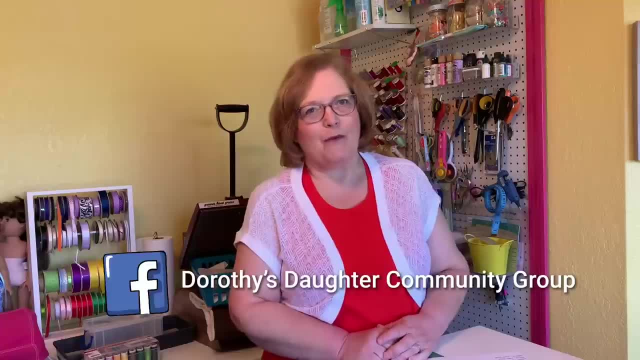 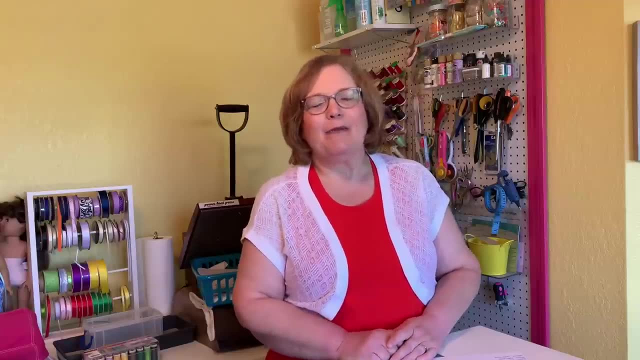 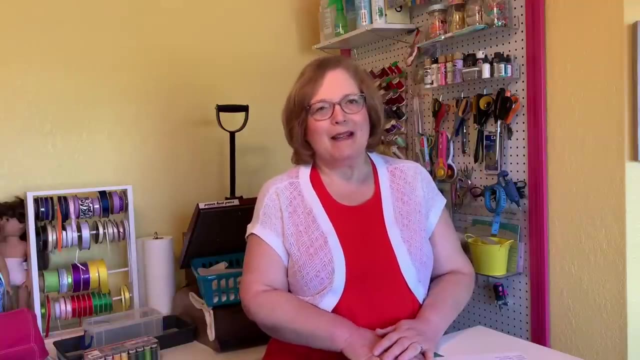 with you my favorite, my top 10 favorite things to sew for kids, Things that I've made for my grandkids or I'm thinking about making for my grandkids. My grandkids range in age from 13 to 3, and we probably will have one more before this is over. I call them my six pack. I have them ages. 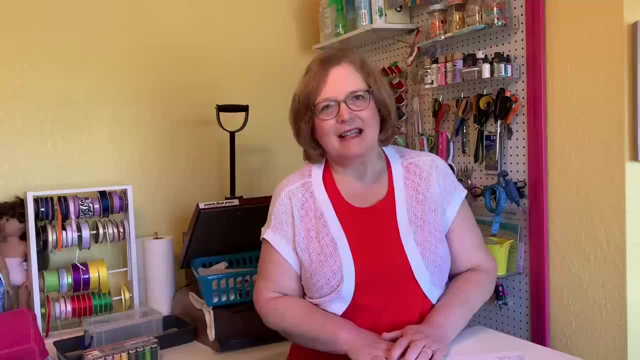 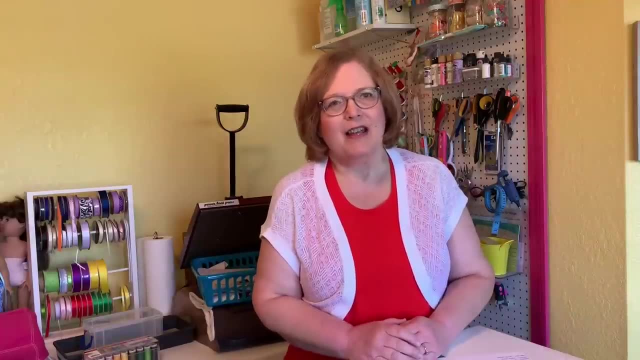 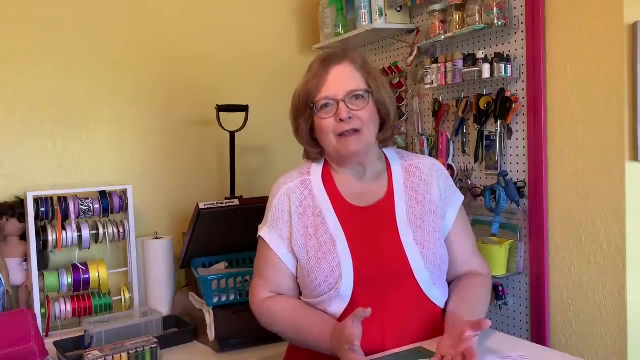 13,, 11,, 8,, 6,, 5, and 3.. So why sew for kids One? it's just a great opportunity for the kids to see how individual productivity can be like, just fostered. I think it's just a really good. 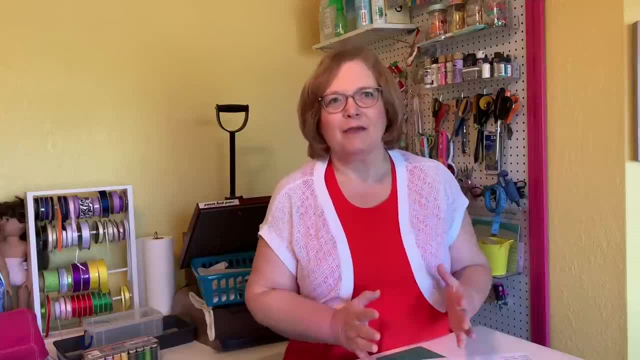 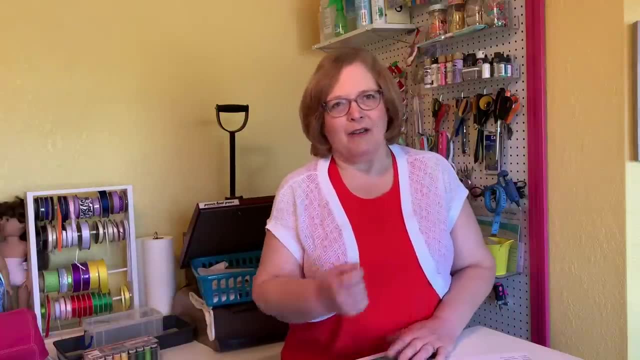 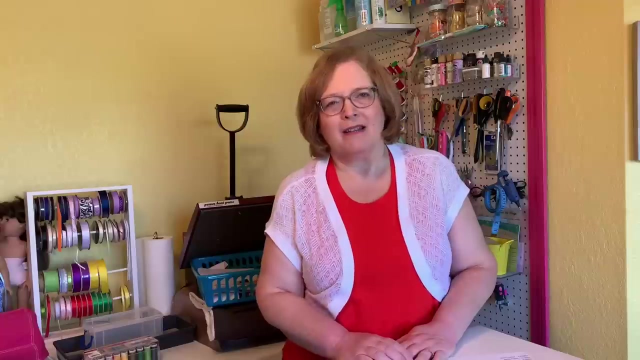 bonding experience. It's special, It's just for them, It's not something you can go out and buy. I tend to stitch love into everything I do and that I pray as I'm stitching. I always tell my grandkids when I make them something and they wear it, it's like every stitch is a hug, So they can. 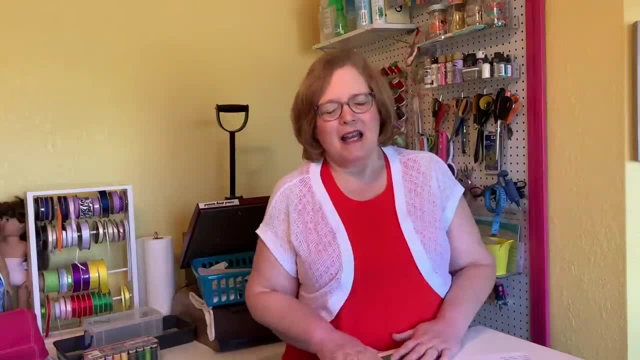 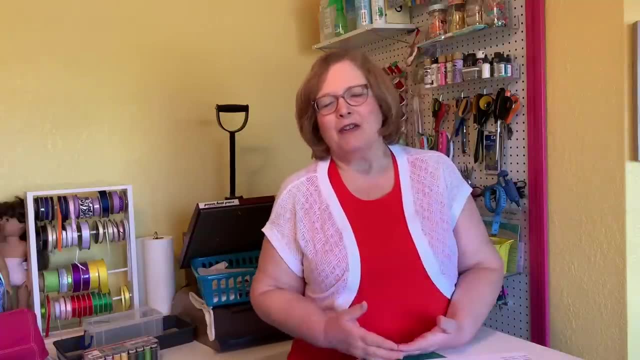 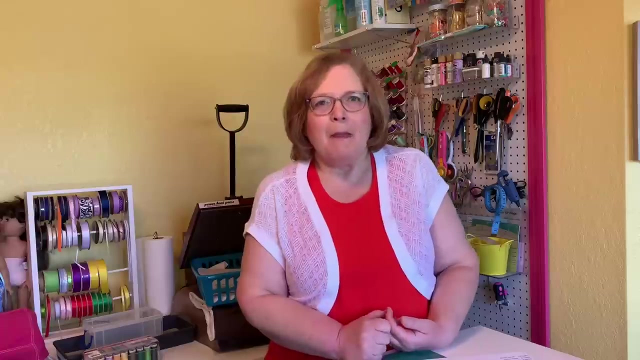 just feel hugged all day long. I just think there's a really high level of love in sewing, A level of special connection whenever you give anyone a homemade gift, but your grandchildren especially. So I'm going to start these top 10 in no particular order, but some most I have made. 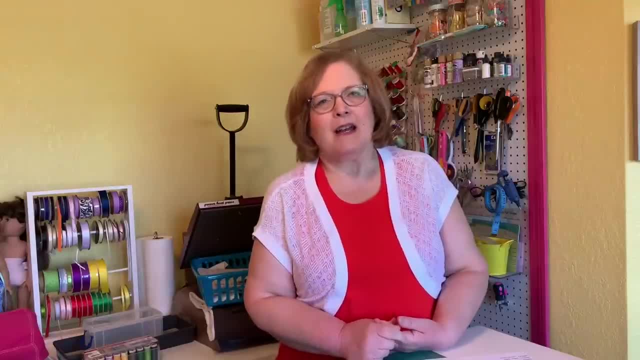 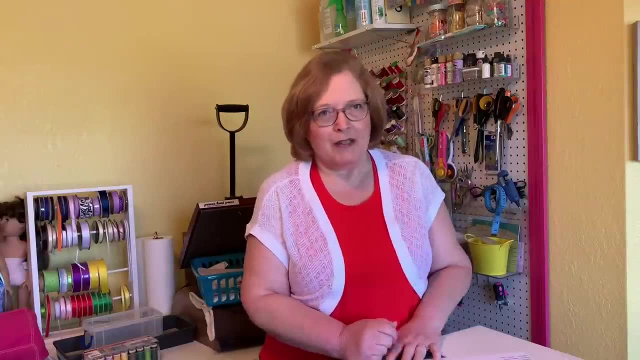 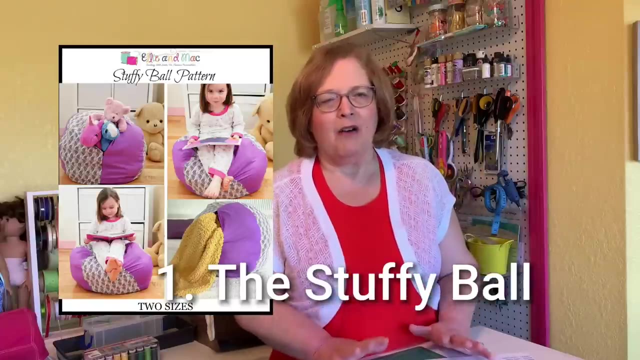 some. I have not only a few, though, and they were just too good to leave off the list. The first one is actually like that Number one, and then, again in no particular order, is the stuffy ball From Ellie and Mac. I have this pattern downloaded right now to make for my grandkids, Actually. 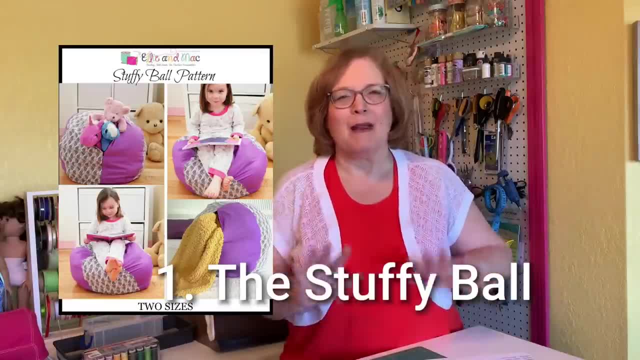 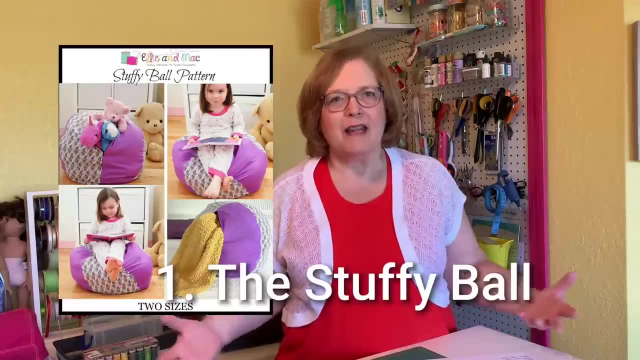 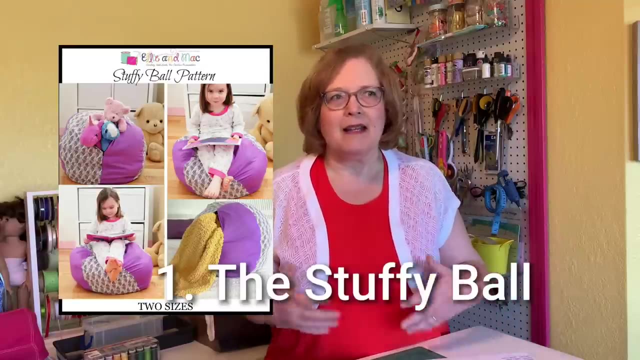 I want to make it for my grandkid room here at the house because we have so many stuffed animals And it's just a great, big oversized ball that you can throw stuffed animals, dolls, blankets, anything like that inside of And it just kind of becomes a place they can flop and 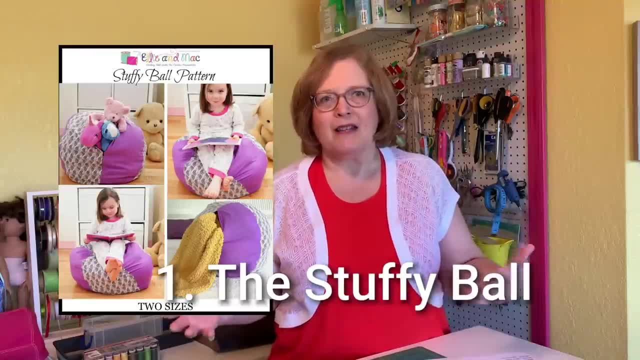 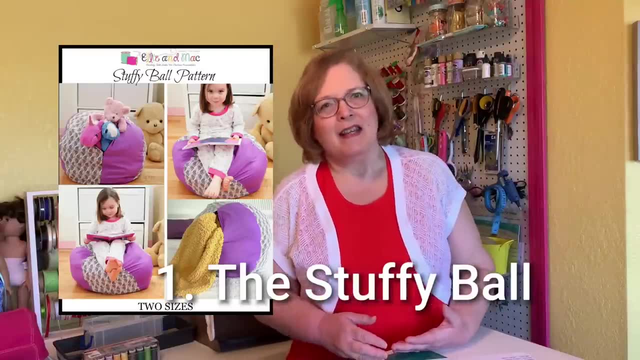 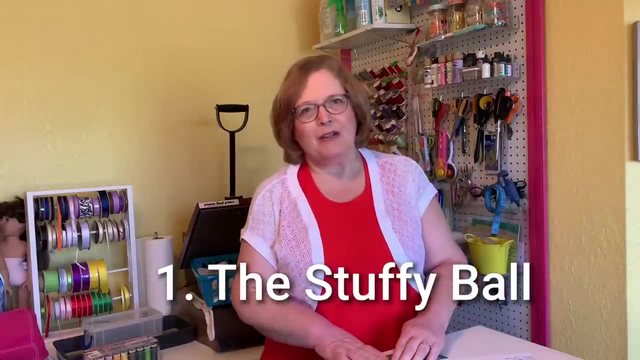 sit, And it also creates a storage area for all those things. I think it's amazing. It's so smart And I think the kids will love it. So I'm going to put all the links to all these patterns down in the description box, So feel free to check those out. 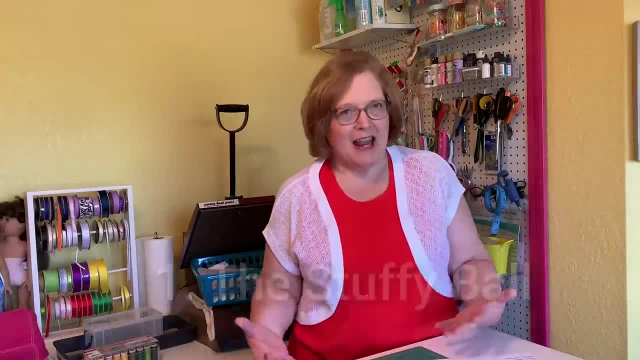 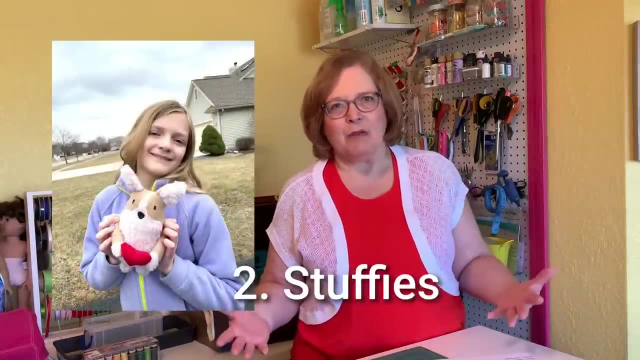 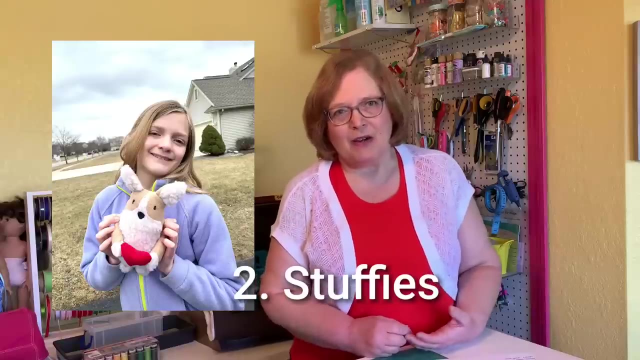 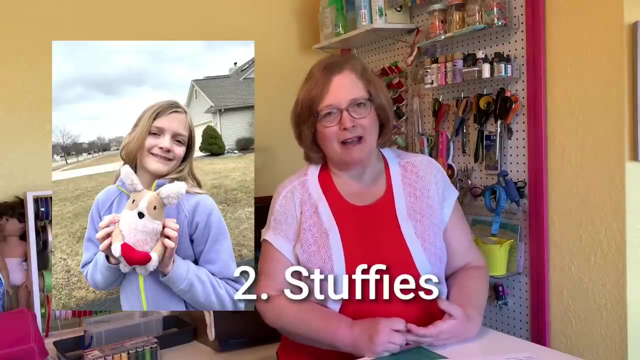 So, as we're talking about stuffed things, the second thing I have for you is actually called stuffies. Now, stuffies are any kind of little stuffed animal that you make for your grandkids. I've made a few of these through the years. I actually have a dinosaur that I need to repair, that I actually made for my son when he was about five, And now I'd like to give it to his little boy. 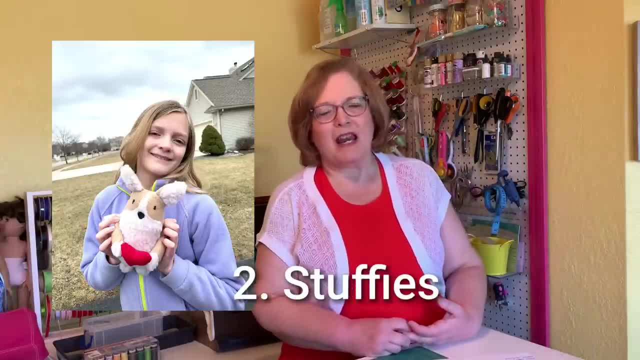 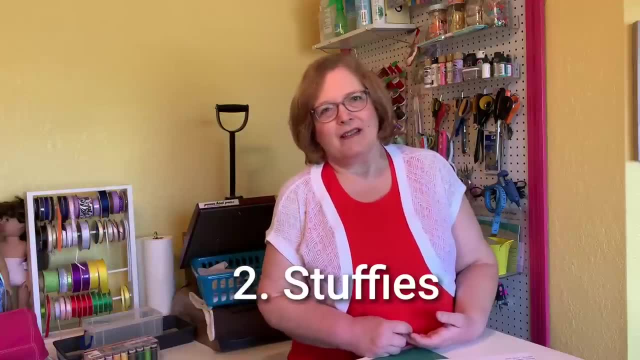 I do have one favorite that I've made. It's Quigley the Corgi. I've made a couple of those. They're fun. I've actually made these with my grandkids. Everybody loves a stuffed animal. I don't really care, I love them. I don't care how old you are, I think you. 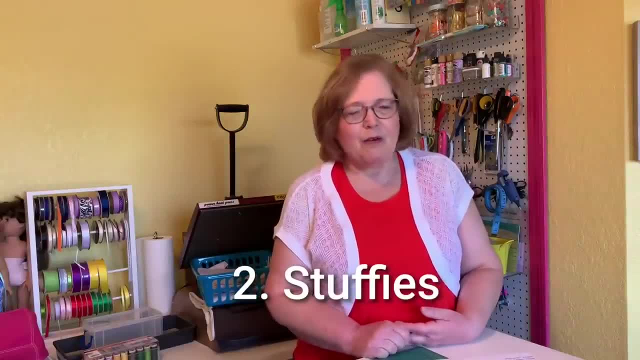 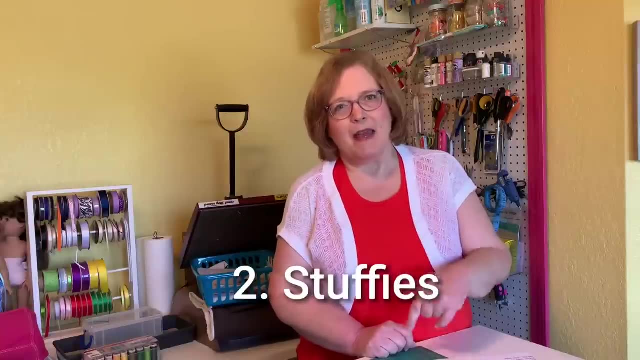 you know, people just love them. So Quigley the Corgi is one, And I am going to put a link below to a site that has over 100 free stuffy patterns. So no matter what your kids' interests are, 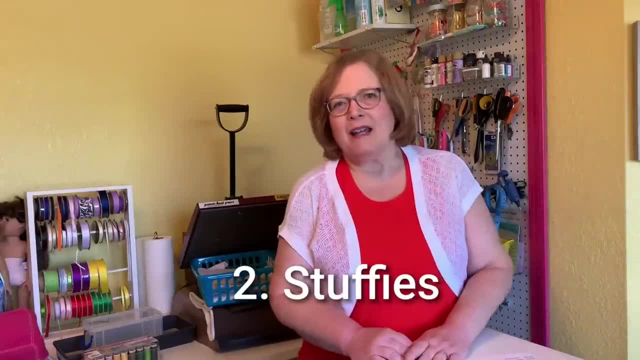 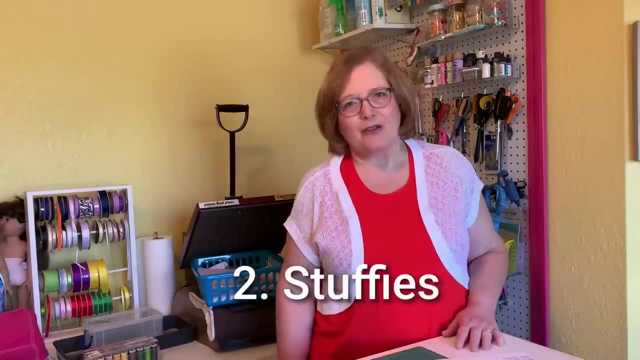 you can find something, So go ahead and follow those links. Whatever your kids' interests are, you'll find a stuffy for it. I think I even saw some of the Marvel characters there. So the third thing on my list are dresses. 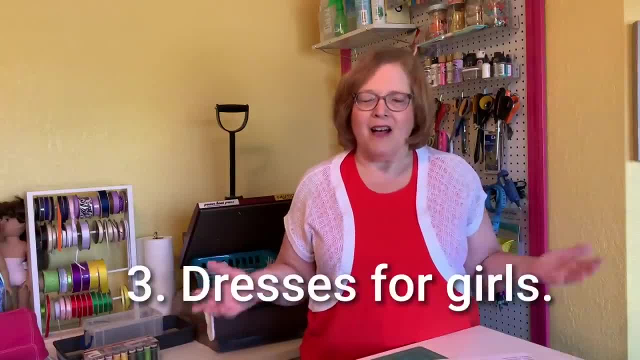 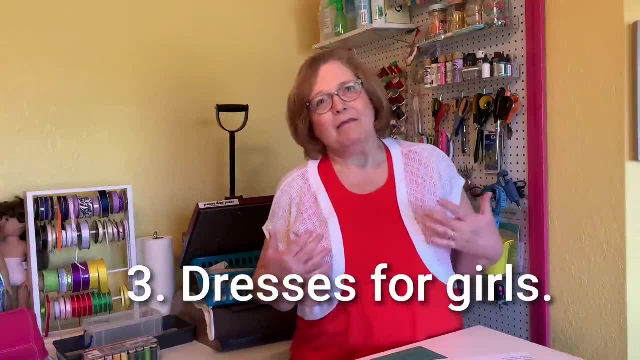 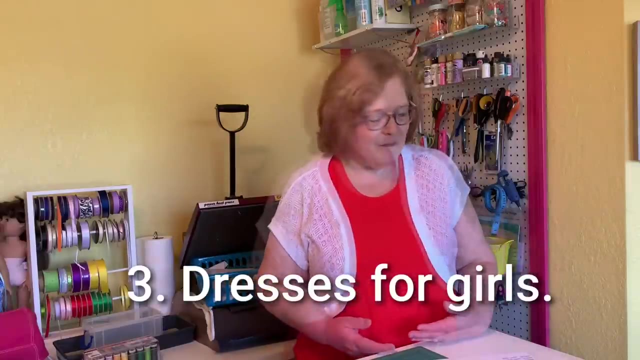 For little girls- What little girl does not love to wear a dress? And I have some favorite patterns. I'm just going to kind of go through the ones that I like. I'm sure that there are more out there. These are just the ones that I've made and enjoy and the girls have loved. One of my favorites is: 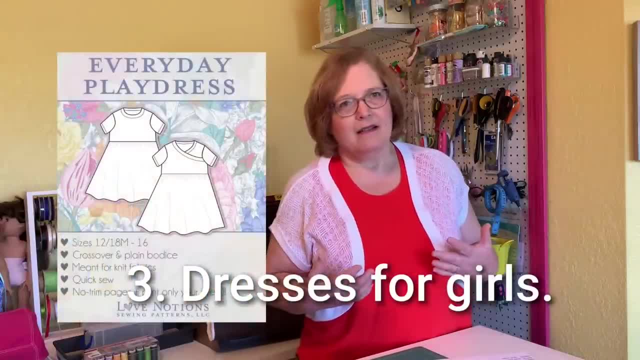 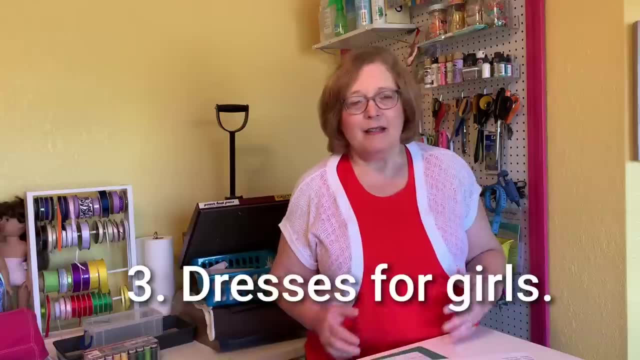 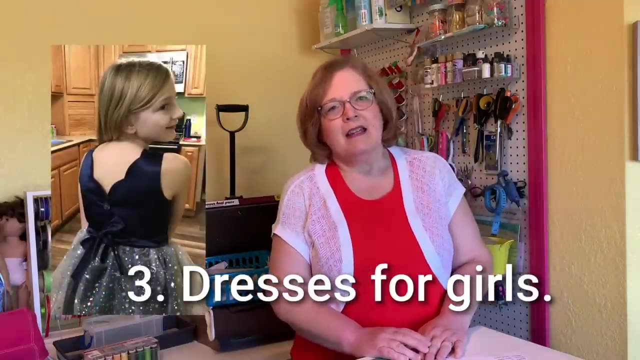 the everyday play dress from Love Notions. I've also made a lot of the Little Lizard King outfits. One of my favorites is the Little Lizard King outfit. I've also made a lot of the Little Lizard King outfits. One of my favorites there is the Miss Haven, which has a gorgeous scalloped back, And the Arendelle. 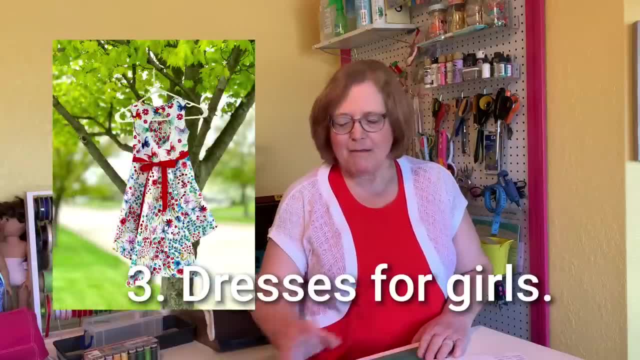 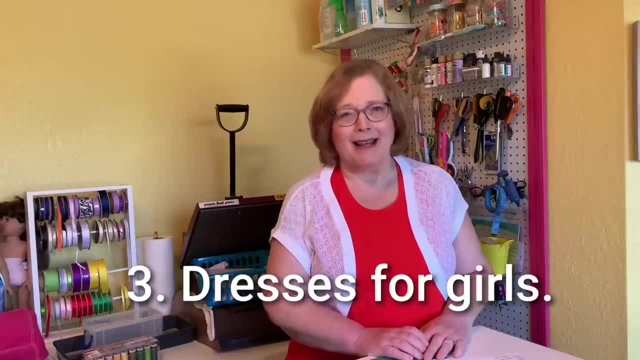 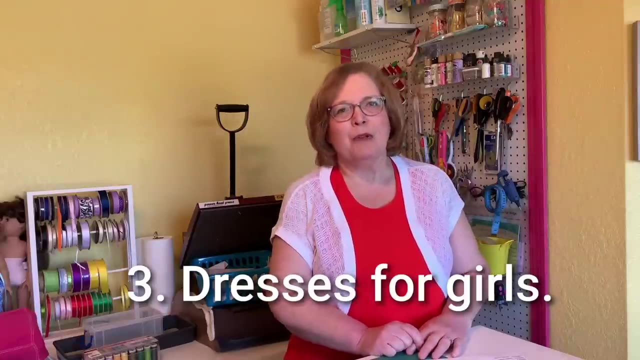 which is very twirly if your kids are into that. My apologies for the background noise. My husband is vacuuming right outside the door, not realizing I'm recording, I think, But hopefully you can hear me over it Also from Little Lizard King. the Bloomsbury dress is just a nice dropped waist knit. 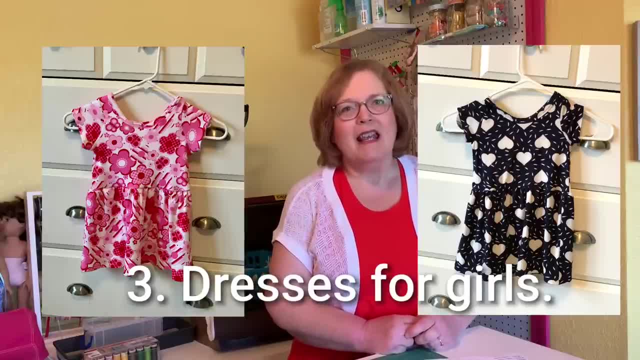 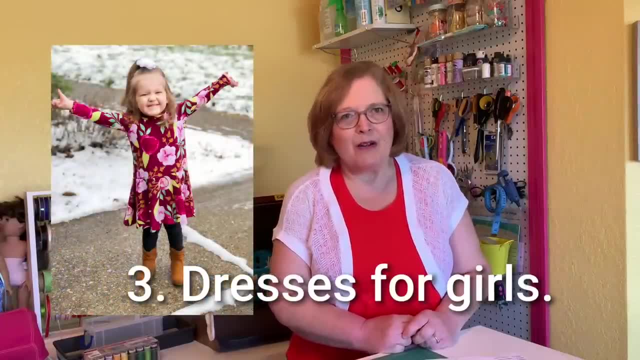 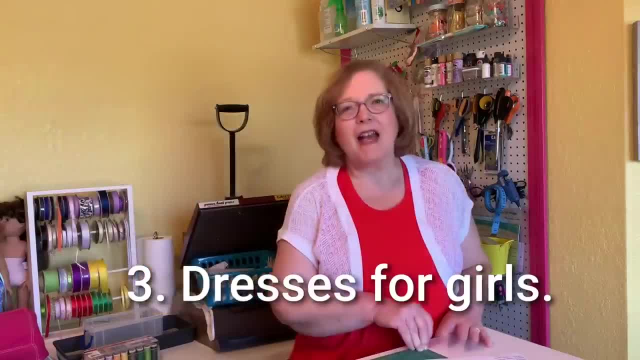 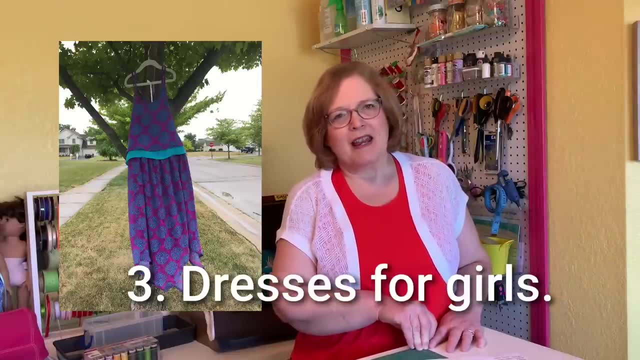 circle kind of skirt, attached or pleated skirt. So that has a lot of options. Cabarita is one that I've made. It's sort of a beachy, flowy, beautiful dress And I've made that for one of my. 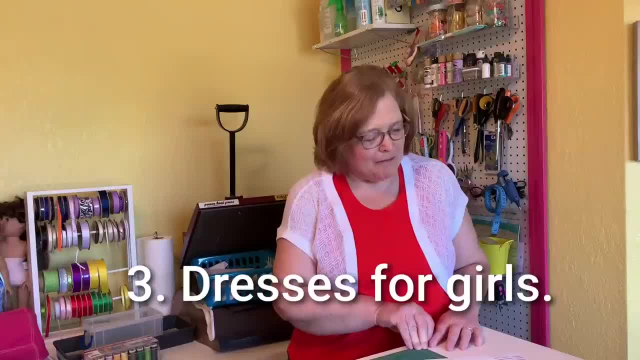 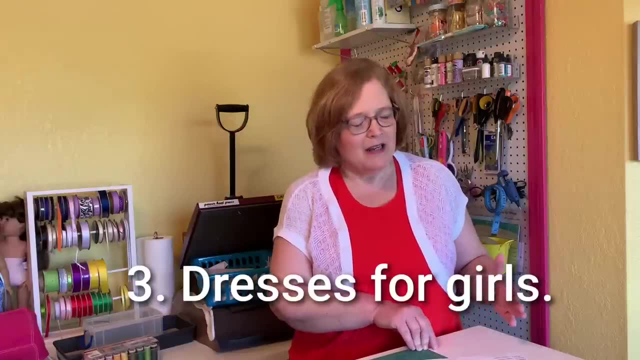 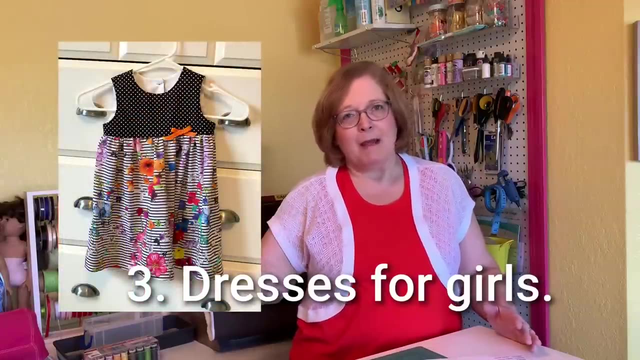 granddaughters who absolutely loved it, And I've made it for my daughter And I've made it for my son. It's very summery. My all-time favorite dress, though, to make for little little ones- It comes in zero to three months, all the way up, I think, to five- is the geranium dress from Made. 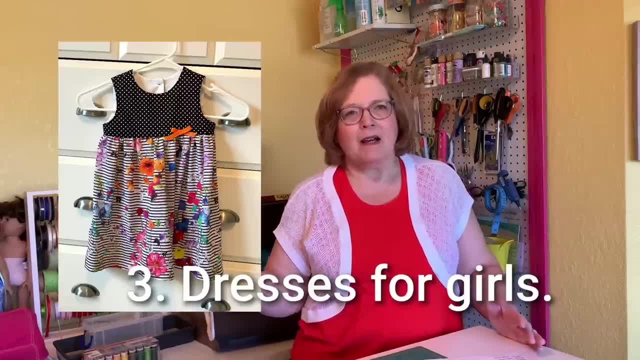 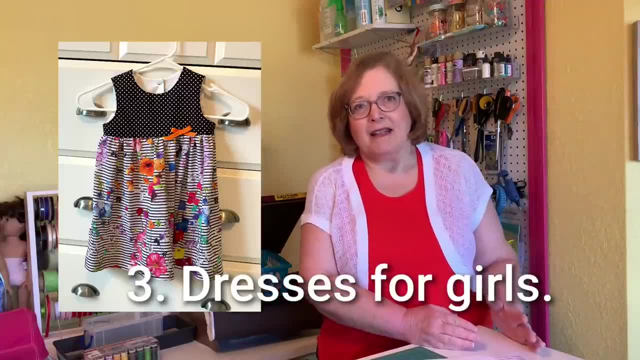 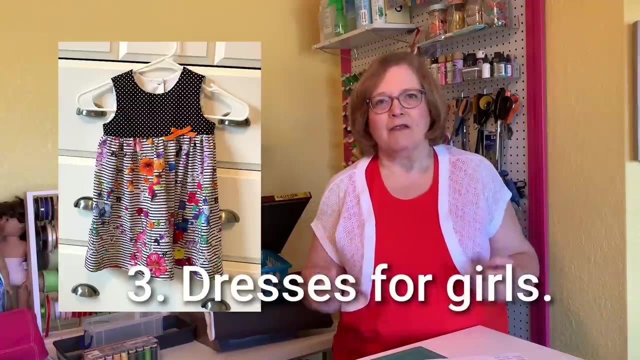 by Ray. Now the geranium dress can be free if you get just the zero to three. I think it's zero to three months- And it's a fantastic baby gift as well, for a baby girl. You can do so many things with it. They have an add-on kit that gives you collars and sleeves, And it's just very versatile. 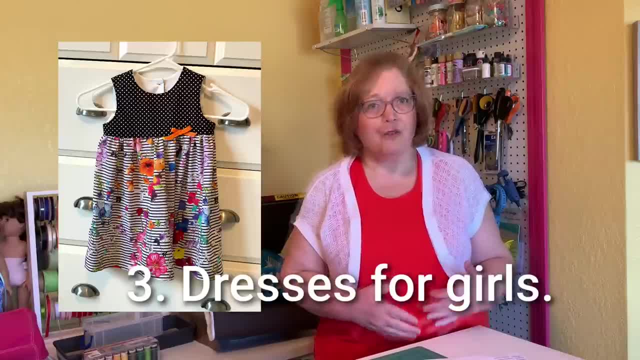 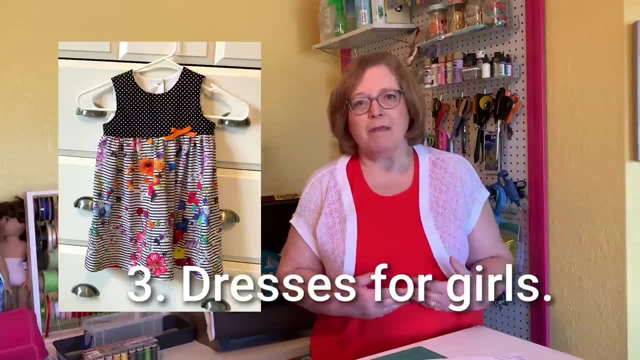 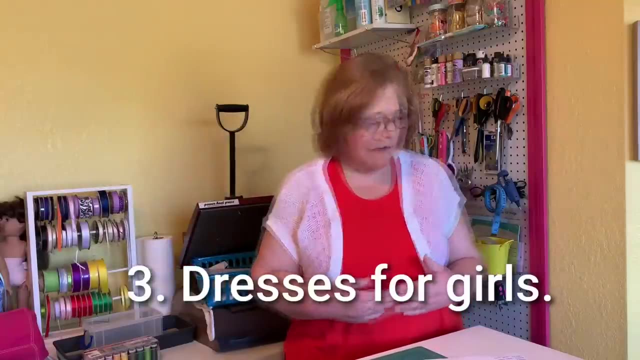 It's a great beginner pattern to start off with. if you're new. It can teach you how to gather a line of bodice- some really basic things. So it's a great beginner pattern to start with And it's my favorite go-to dress pattern for really small little girls. Number four are boys' dress clothes. 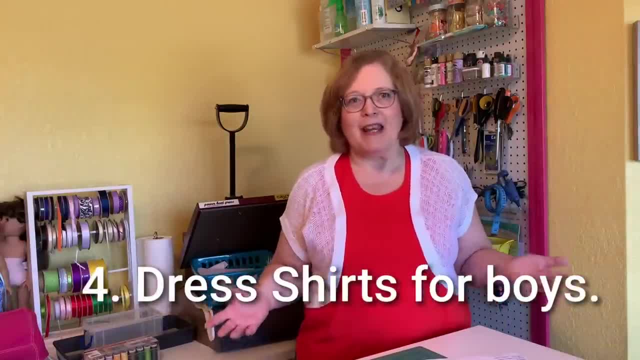 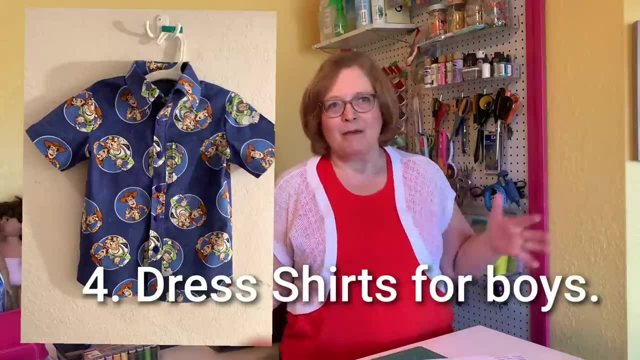 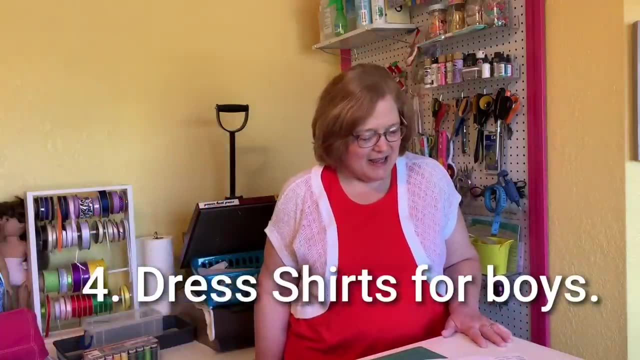 You can't leave the boys out, So I've made shirts for my grandkids, I've made shirts for my aunts. One of my favorites was this Toy Story shirt that I made for my grandson when he turned four. It was right when Toy Story 4 was being released and he just loved it. This was Simplicity. 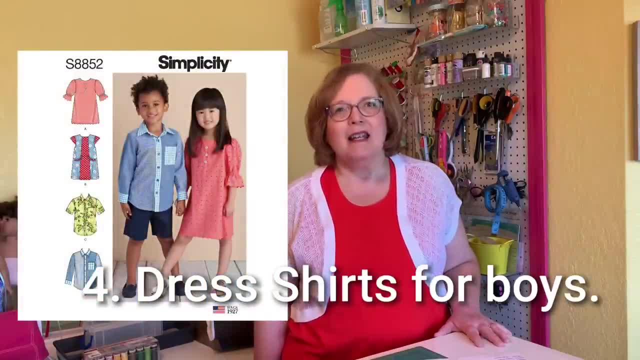 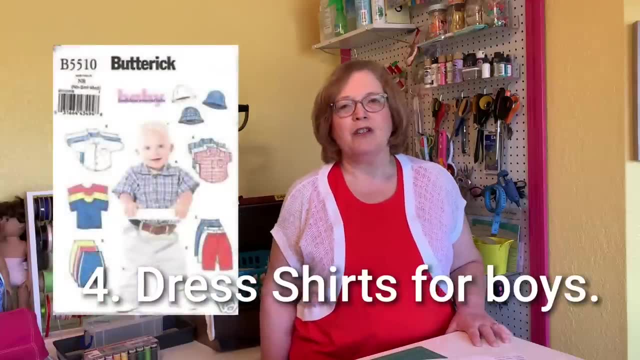 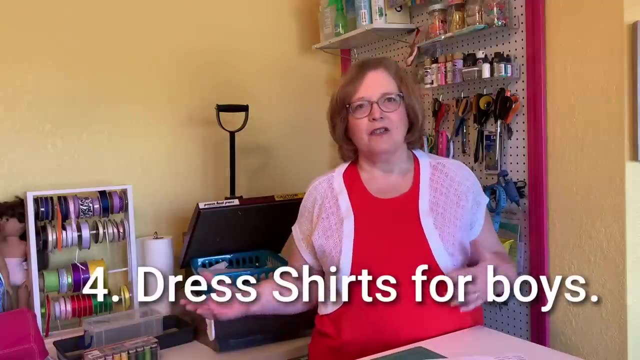 8852,, which goes from sizes three to eight. I've also made the baby one that is Butterick 5510, and I've made a larger one that is McCall 6222,, which is youth boy sizes. It's actually a. 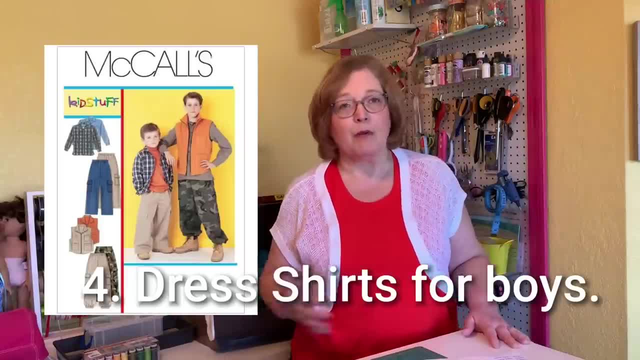 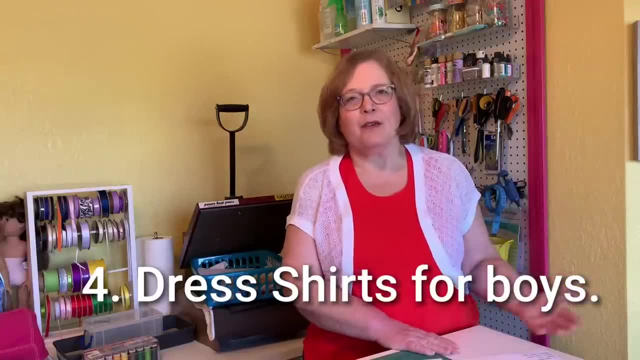 Daddy and Me type pattern. that is really kind of cool. It's for both men and boys. Dress shirts are always fun, but you can also make flannel shirts Again, just like I did with Toy Story. you can make their favorite character a sports team, just an Easter outfit. Make a. 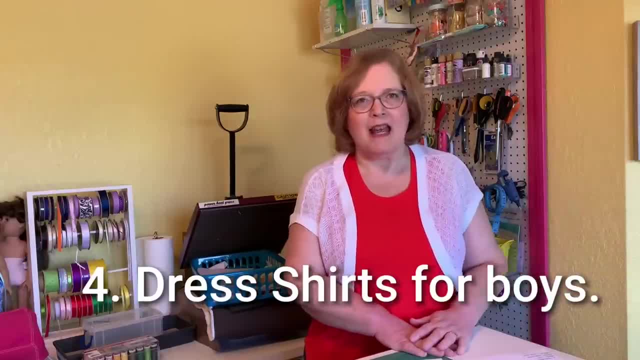 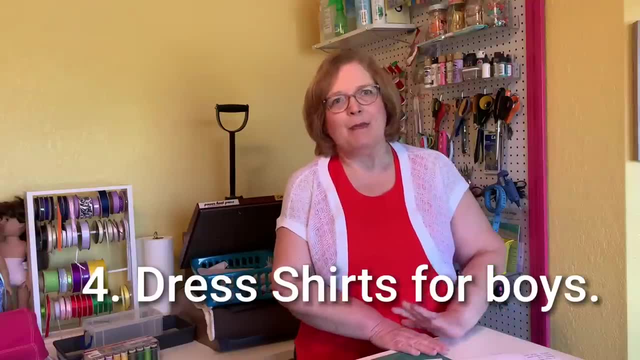 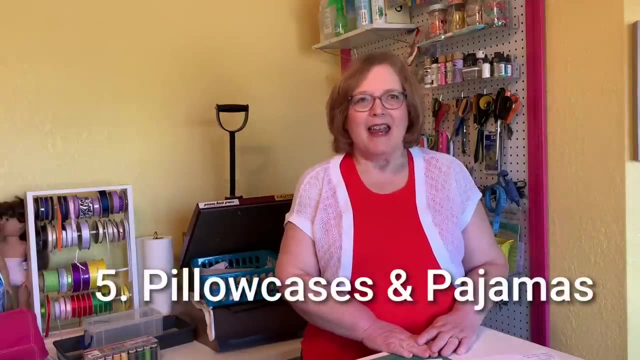 little bow tie to go with it and you've got a fantastic dressy outfit for a wedding, wedding or anything that you can imagine. So that's number four would be dress shirts for little boys. Number five super simple idea here is- and this is a great thing to take to a kid's 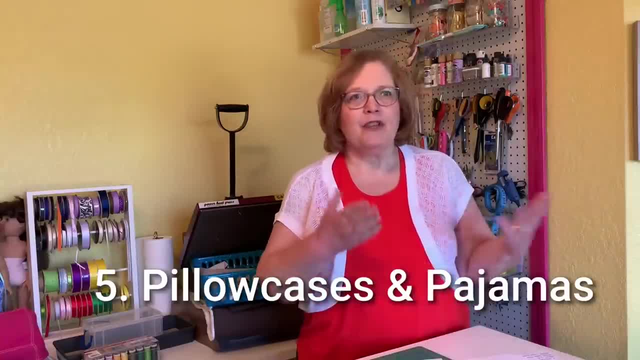 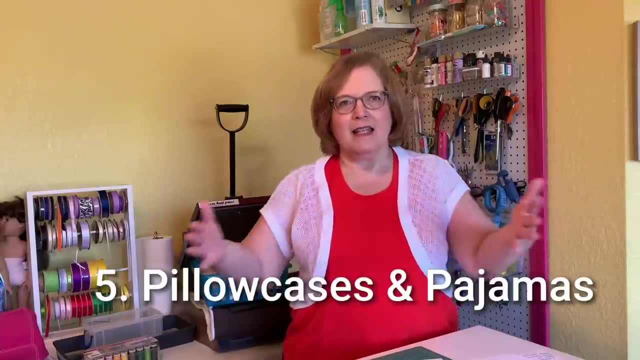 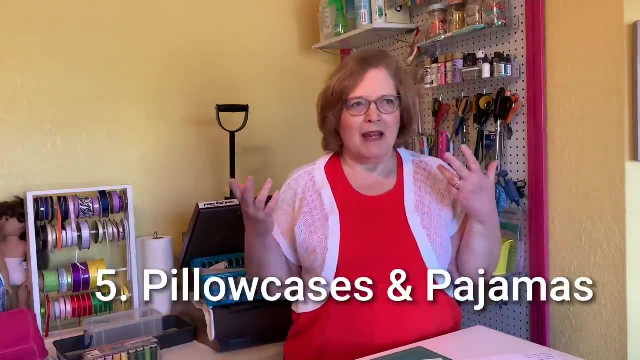 birthday party pillowcases with jammy pants or other jammies. So number five would be nighttime related things: jammy pants and pillowcases and pajamas. So my favorite thing to do is to make a character's pillowcase and then make some. 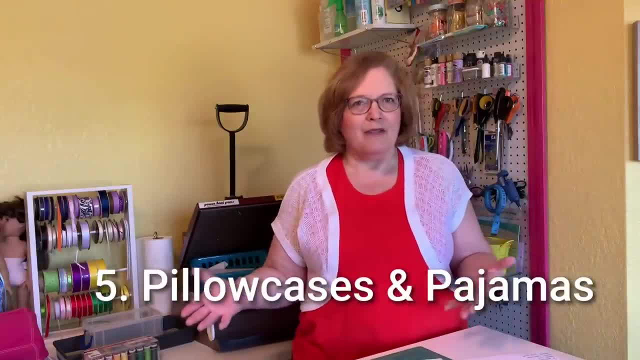 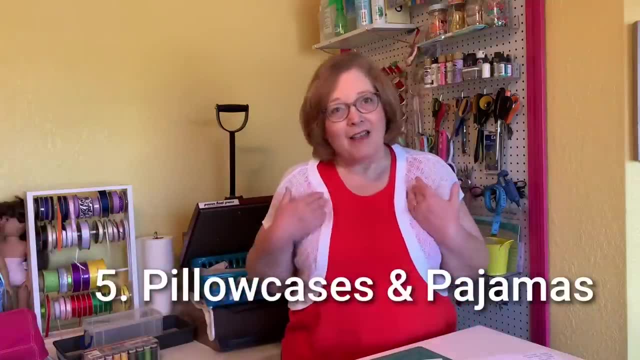 jammy pants that match it, And it's a wonderful gift to give. You can give that to all the way from three years old all the way up to you. know, teenagers even love it. I love it. I made myself a Mickey Mouse pillowcase and I love it, So it's really for all ages. 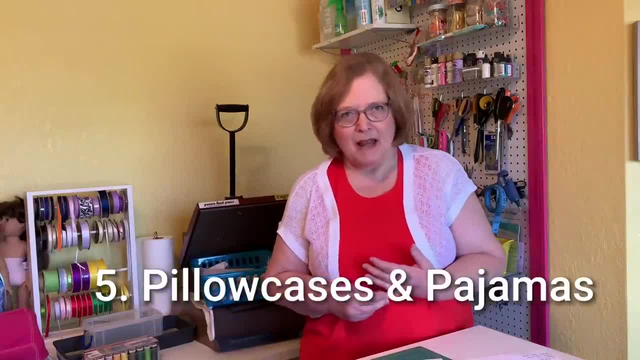 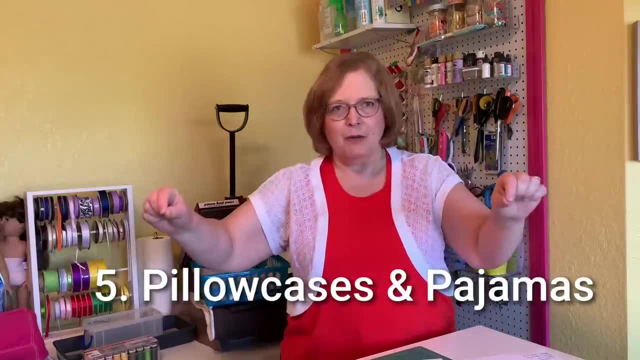 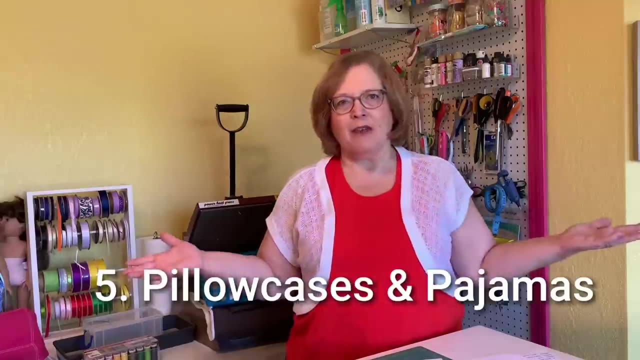 My favorite patterns here. pillowcases don't need a pattern. You basically take 34 inches of fabric, You sew it in a tube, You sew the end shut, You fold over the hem three inches and you've got a pillowcase. It's fun to learn with. It's fun to make with your kids. It's also. 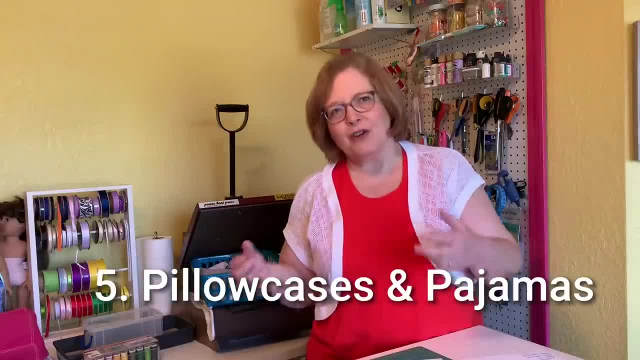 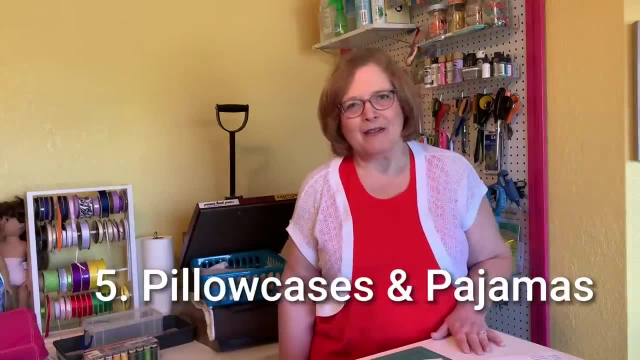 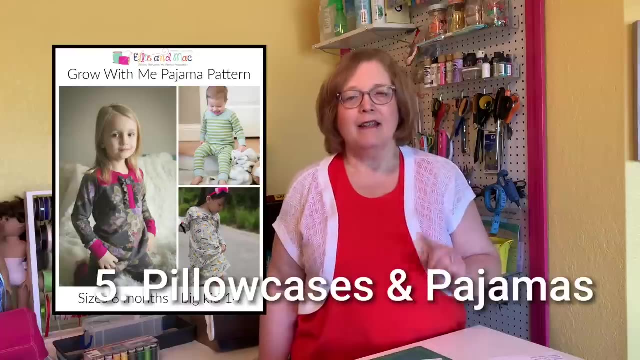 a great thing to use French seams on. If you don't have a serger, you can go ahead and do French seams, and they turn out really, really nice. Two other jammy patterns that I love are the Grow With Me jammies from Ellie and Mac- A free pattern, may I add, and it's wonderful. 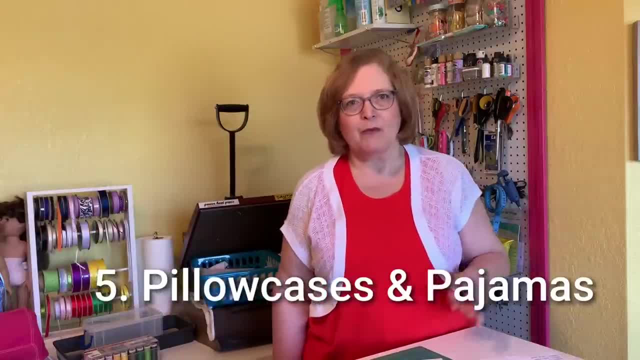 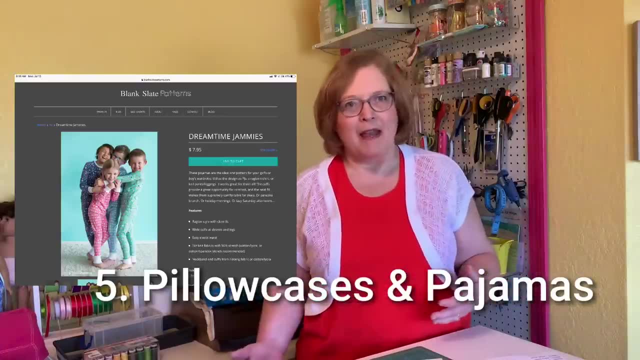 Walk the Plank. jammy pants from Patterns for Pirates, which also is free. Dreamtime jammies from Blank Slate Patterns, which is connected with Melly Sews. That's a great pattern. I've used those for Christmas jammies several years in a row And also the Movie Night jammies. 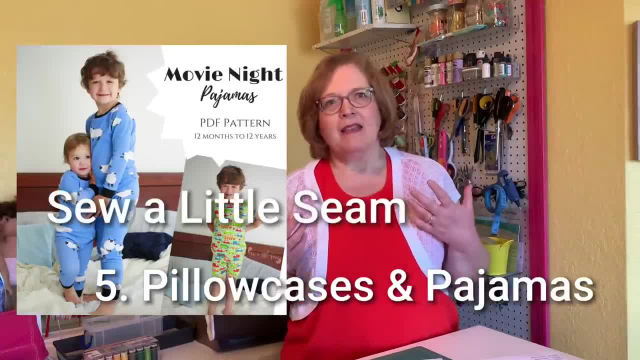 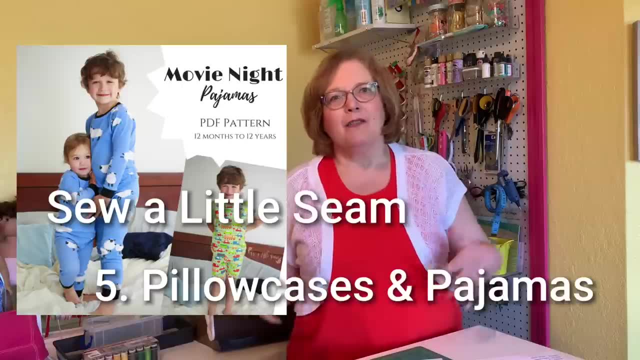 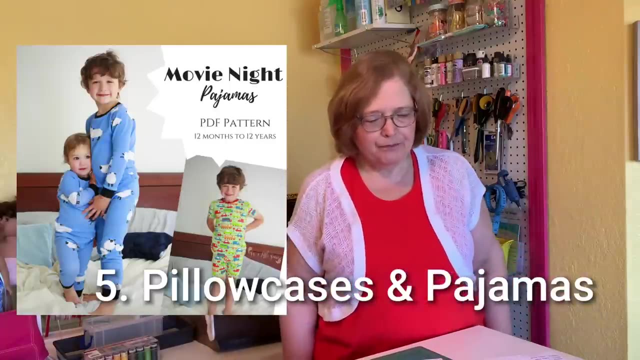 and they're from Stitch Upon a Seam And they are fantastic Patterns and they go all the way from really small to adult. So if you're looking to make like a whole family full of Christmas jammies, that is a great go-to pattern. The Movie Night jammies. 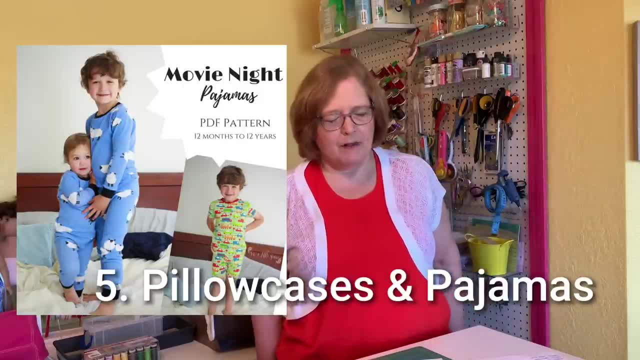 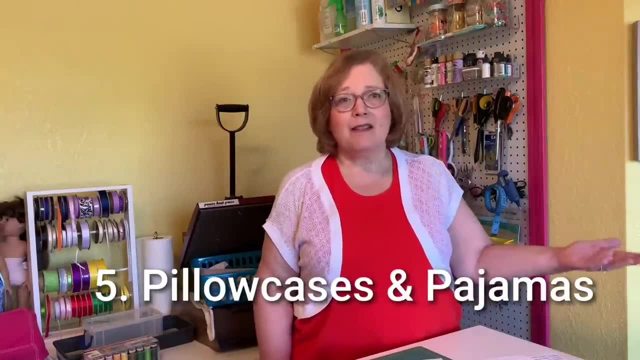 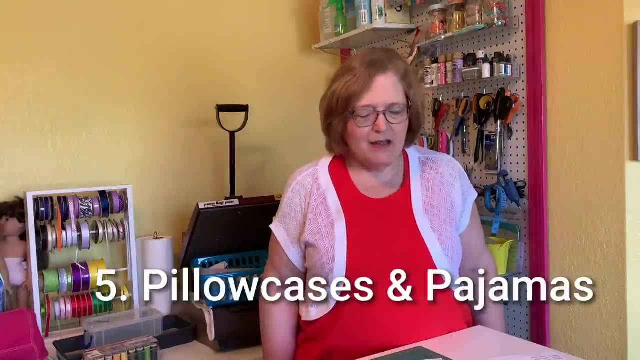 I believe if you join their Facebook group are free as well. So lots of fun coordinating pillowcases and jammies or even a stuffy and jammies. You can combine things on this list and you can do a lot of different things, So it's a great way to personalize gift. 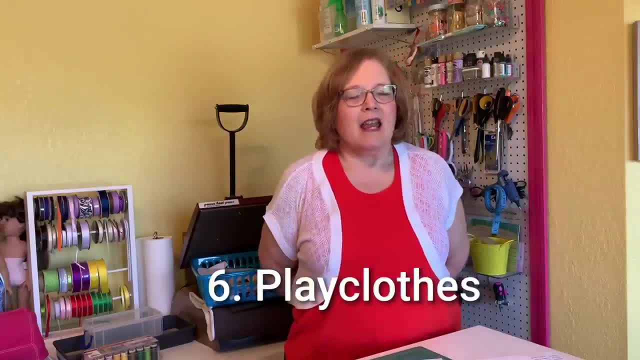 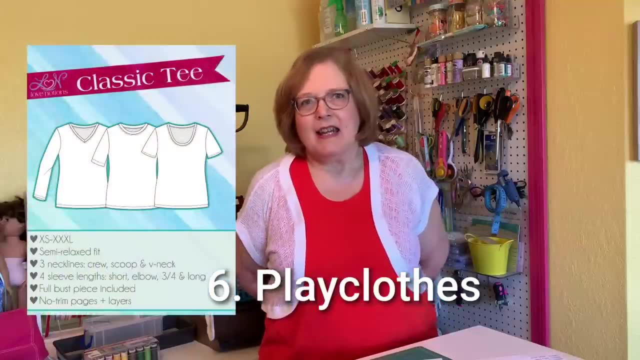 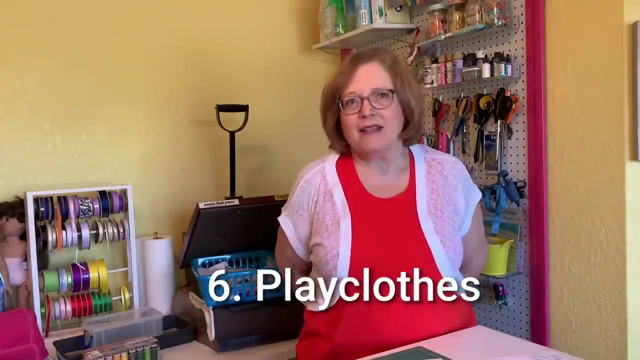 Number six is play clothes. Many of the designers have tons of different tees and shorts: The Bee Active shorts from Ellie and Mac, The classic tees for kids from Love Notions. There's also rompers. My favorites are the South Shore romper from Ellie and Mac. 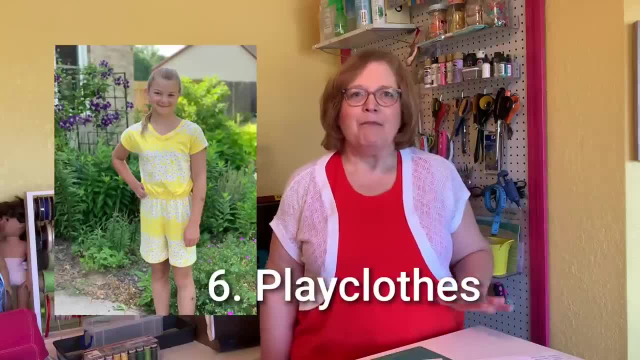 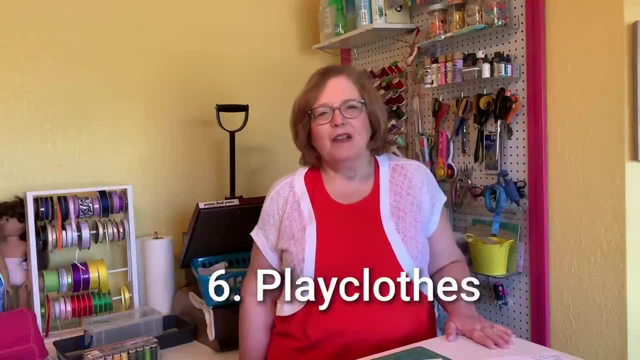 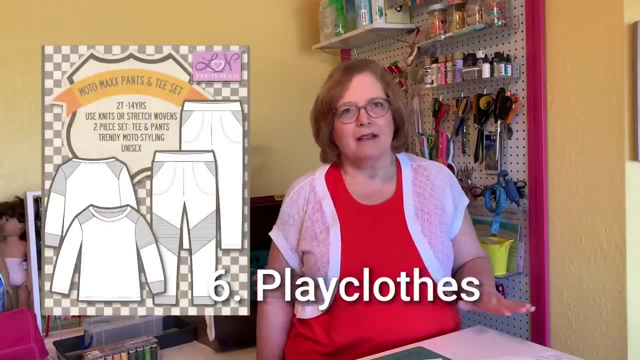 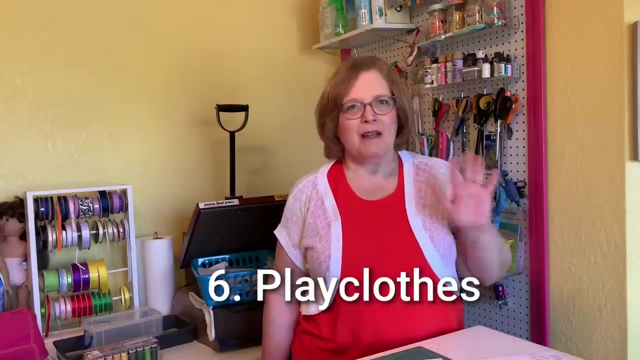 Also the Sunday romper which is new from Love Notions, Also the Isla romper from Little Lizard King. But play clothes make a wonderful gift. If you're looking for fall, there's the Moto pants from Love Notions. Ellie and Mac has too many to mention of kids play clothes. I mean you can. 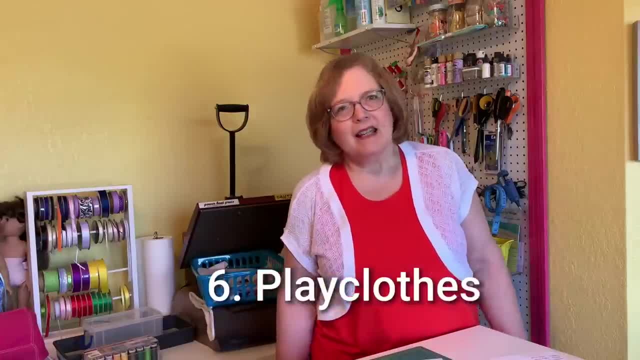 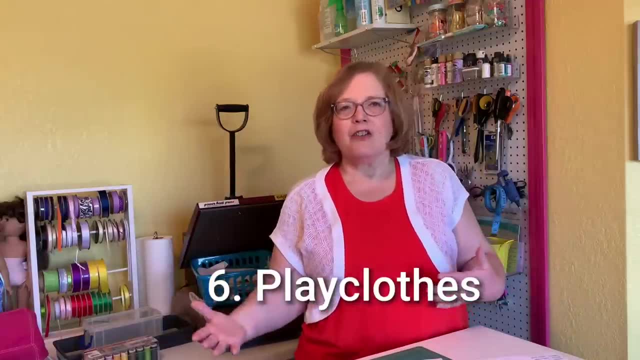 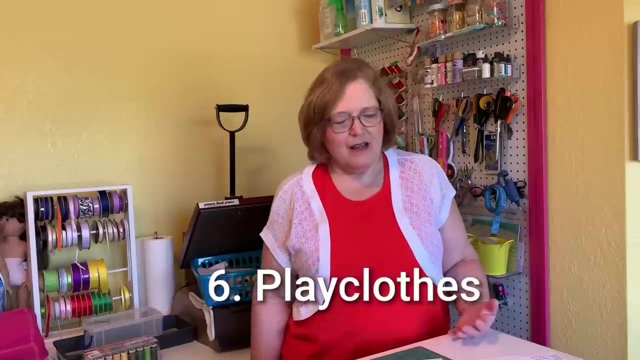 there are just so many patterns, Um. but Kids love things like that, and if you can combine it with their favorite color, their favorite sports team, their favorite character, you can come up with a really great personalized gift for them. Number seven is a backpack. Now, if you've watched me for very long, 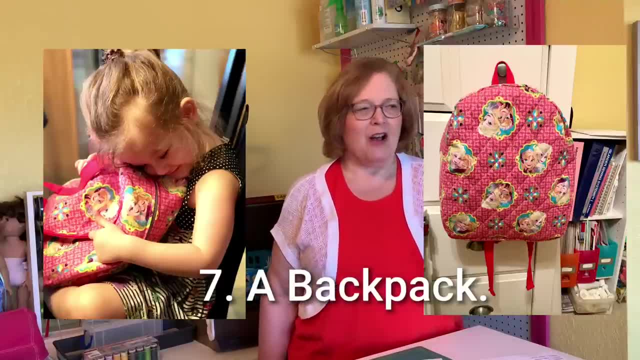 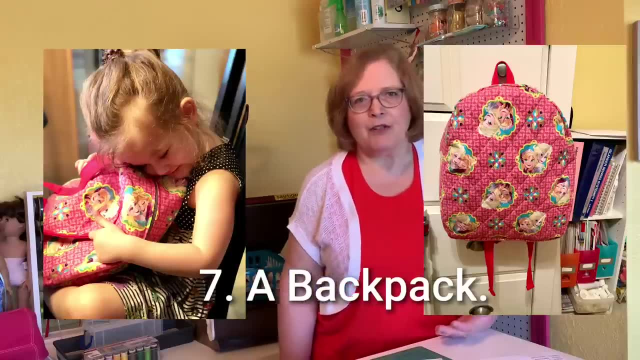 you know that I've made several of these for my grandkids. They all get one right about the time they turn three or four, And I use the Toddler Backpack, which is a free pattern from Crazy Little Projects, and I'll put the link down below. 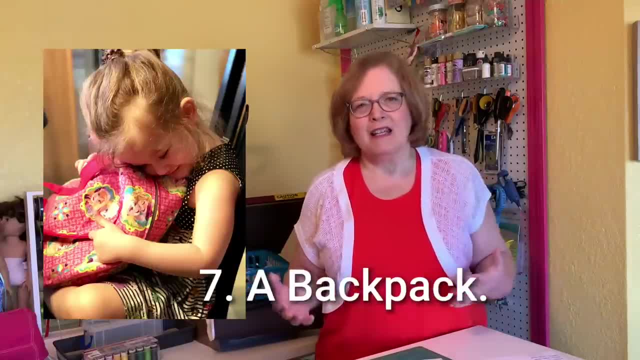 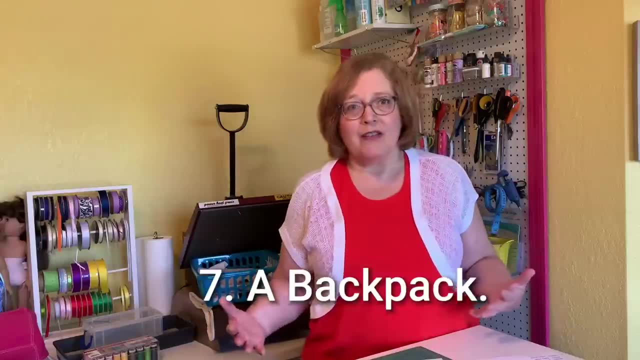 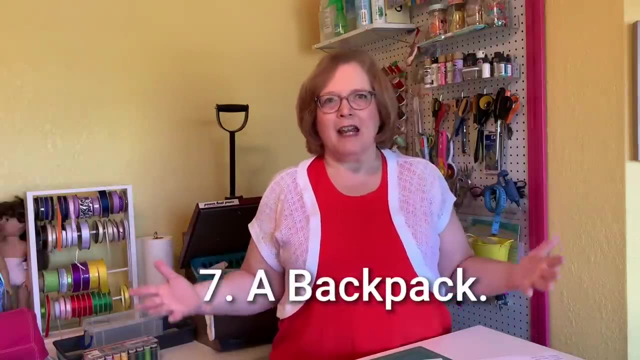 It's fantastic. It's a very quick sew. The kids have all loved them. You can use any quilting cotton that you like, including the characters, So I've made them anywhere from the Good Dinosaur to Toy Story to Frozen. I have done the gamut in these and they are wonderful. 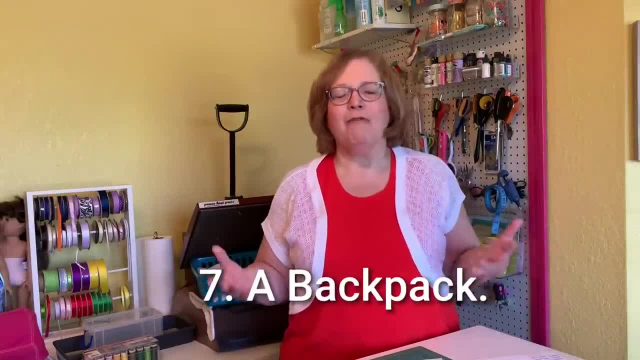 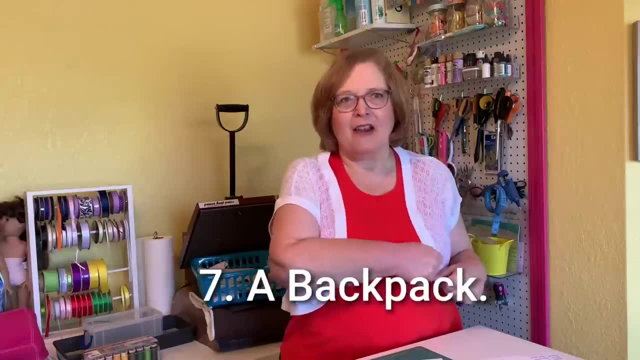 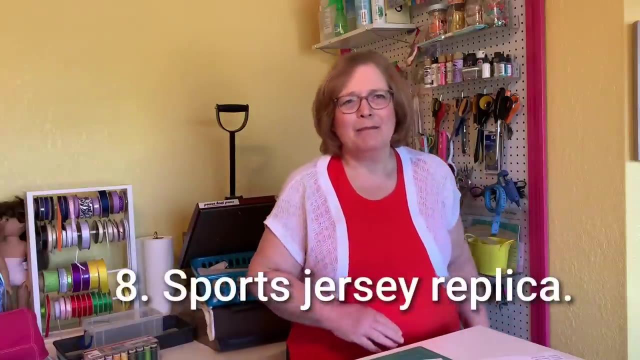 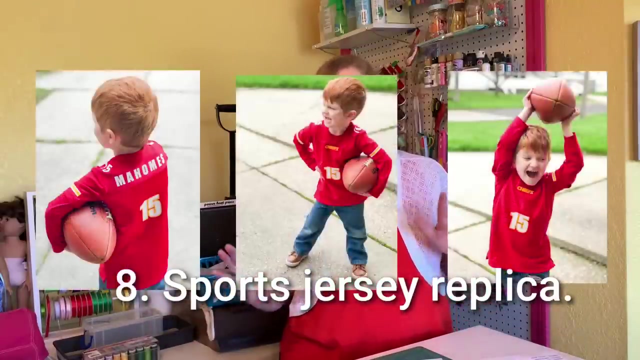 Kids love them. Kids love bags. I think they just love having their stuff in their bags and they carry them around and it's, it's incredible, They love them. Number eight sort of falls into the play clothes category, but it also deserves its own mention. Number eight is the game day jersey from Love Notions. 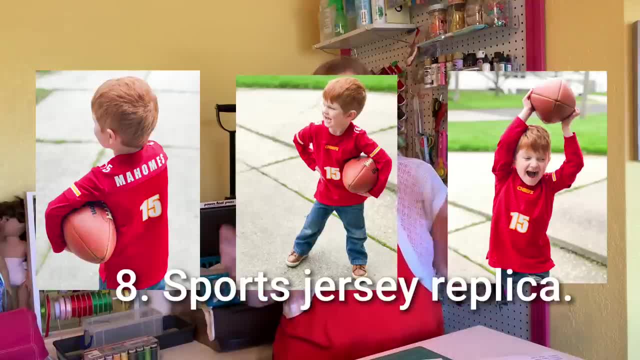 Now I have taken that pattern and I have made a very official Kansas City Chiefs jersey. So if you take that pattern and you look at their favorite team, you can go ahead then and put whatever numbers on there with vinyl, heat transfer vinyl or you know, embroidery if you have an embroidery machine, or applique- however your method of choice. 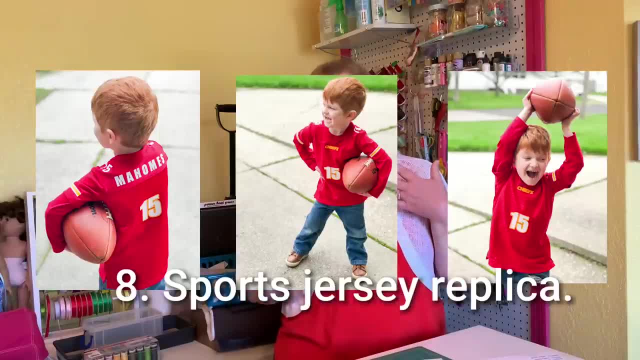 But you can turn that into a very authentic sports jersey. I did a blog post for Love Notions about this and I'll put the link to the blog post down below. Athletic mesh can be hard to find. I did find a really good supplier for it and surprise. 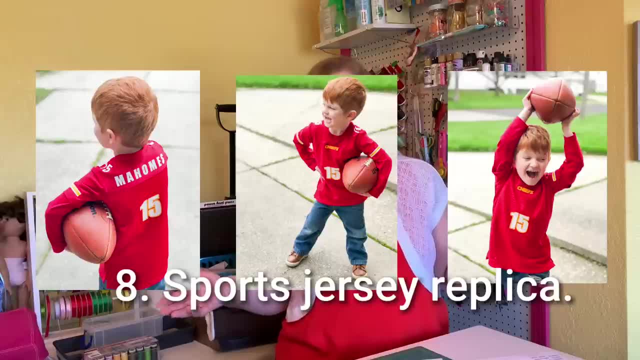 it's only like $3.99 a yard- regular price, So it's really affordable, and I found, though, that you need to kind of line it, because it just- the holes- make it kind of a flimsier fabric without a little bit of support behind, But I just lined it in. 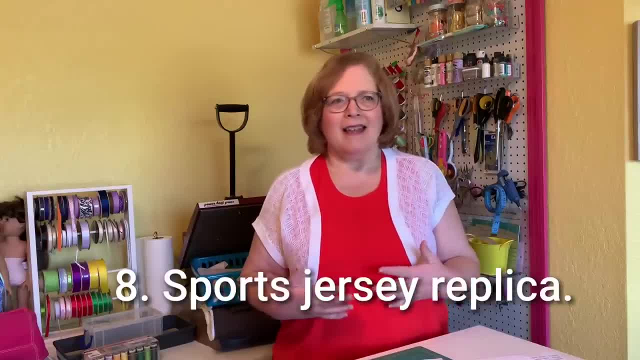 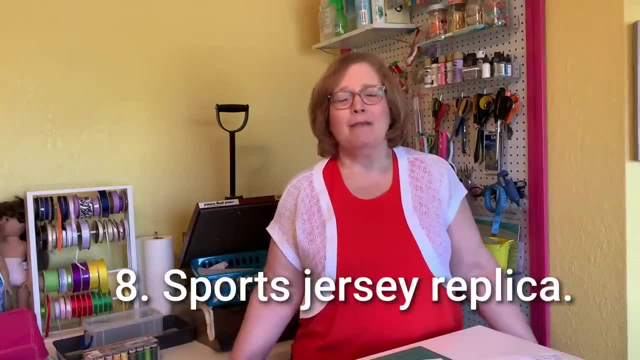 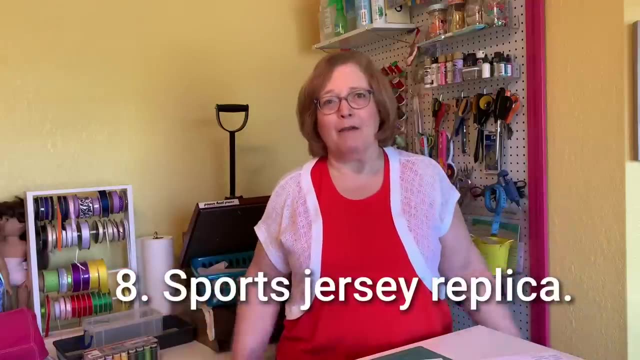 some red cotton lining. It's a little micro that I had and it was. it's just so cute. So if your little ones have a favorite team, you could even make it Team Mickey or Team Donald or Team Anna or Team Captain Marvel, whatever. 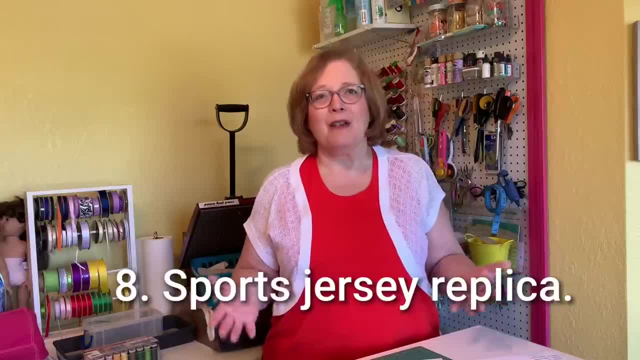 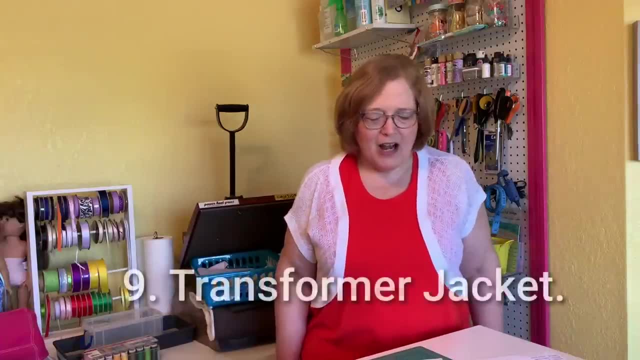 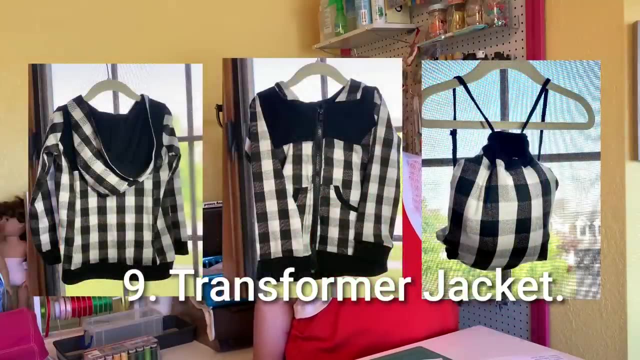 You can just personalize it to whatever their favorite thing is and you can make an authentic little tiniest sports jersey ever. All right. number nine is the Transformer Jacket from Ellie and Mac. Now, this is a wonder, this jacket. In fact, I want one. 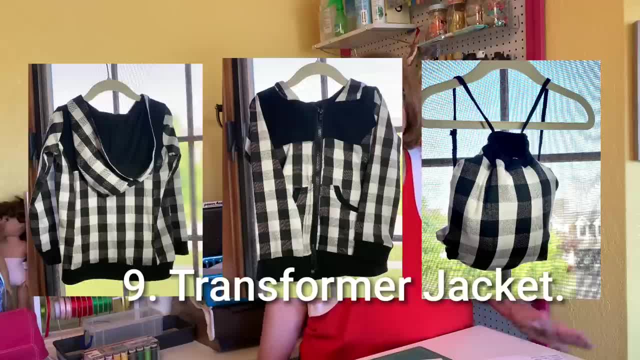 I'm going to make the adult version for me. So it's a jacket, a hoodie that turns itself into a backpack that you can put on your back, and you think, okay, yeah, but why? You wouldn't carry anything in it, because you might wear it as a jacket. 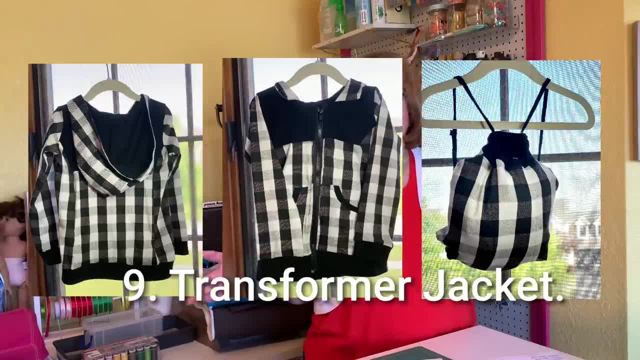 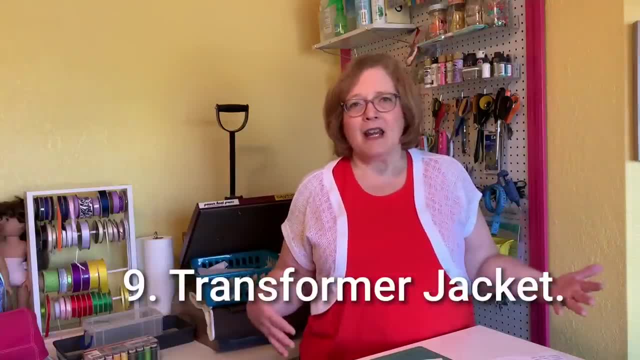 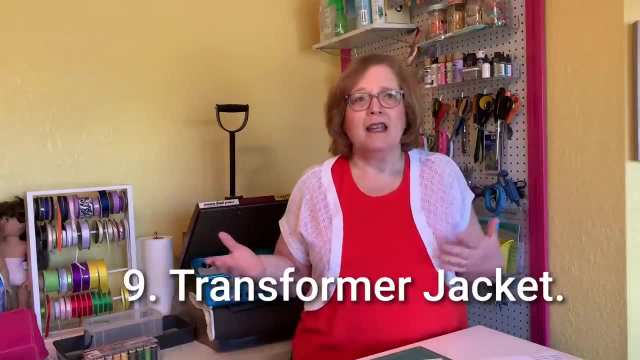 You know, I tossed around why and then I realized that here in Ohio we have days where it's warm all day long and then in the evening it wears off and is really cool, especially if you go somewhere like Cedar Point or to the lake, and then it gets cool in the evenings. 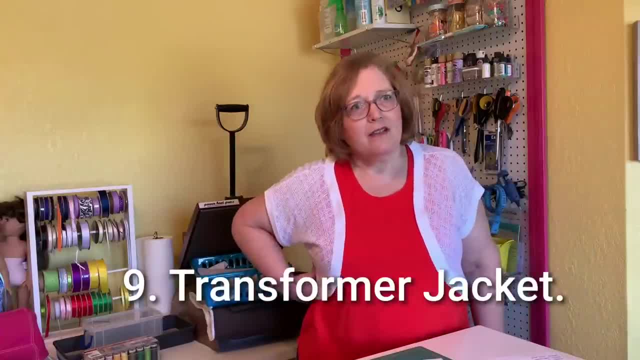 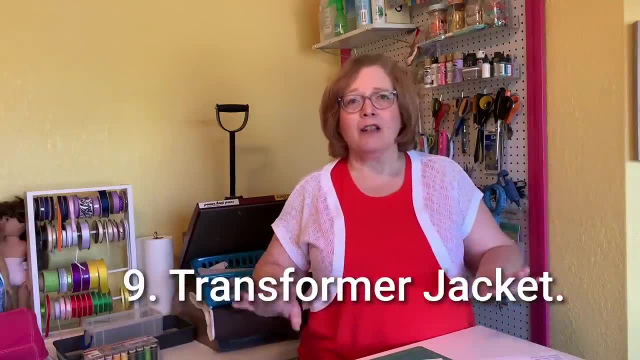 So instead of carting all of your kids' jackets to the lake, you can just have them wear their jacket. You could walk around Cedar Point all day long with your jacket on your back, ready to put on when it gets cooler outside- and I know there are a lot. of places where it gets cooler at night. If you live in the desert- I believe it does Here in Ohio- if you're by the lake or the river or anywhere like that, it will always cool off at night. Different times when we've done a Cedar Point day: 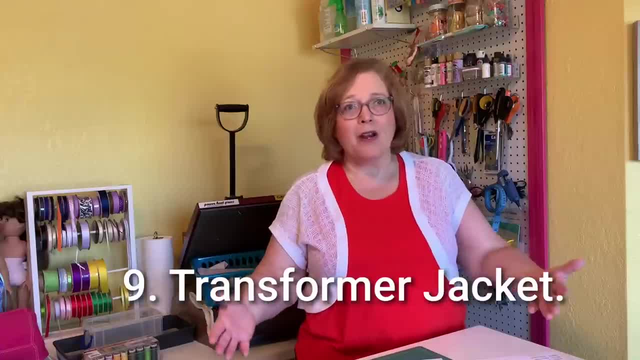 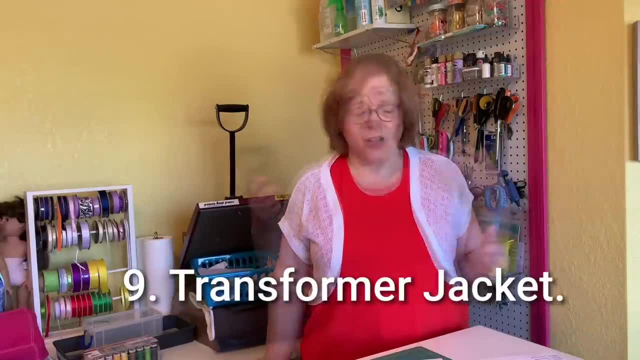 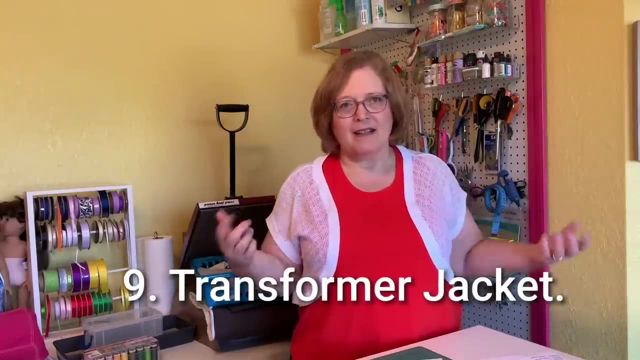 having a jacket has been a real problem, because where do you put it all day? So this is a great option for just carrying your own jacket all day long. So I want one for airplane travel, Because if you wear it when you're going through security, it doesn't count as carry-on. 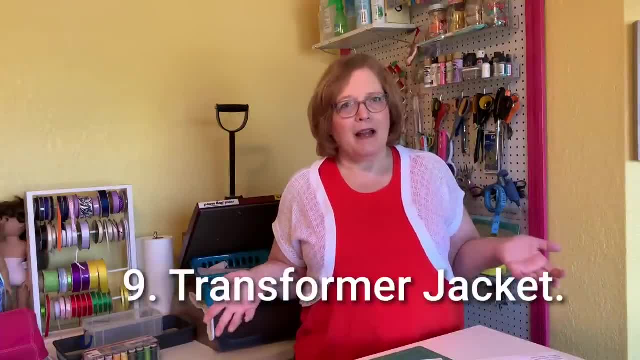 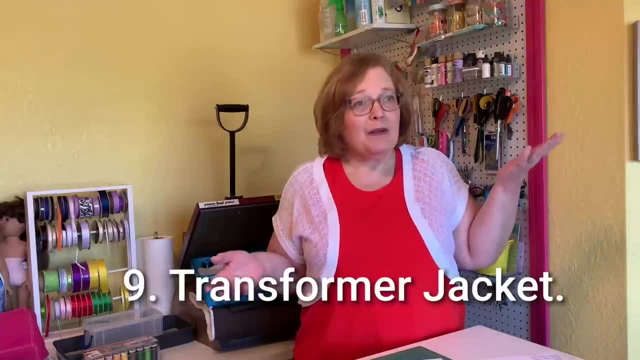 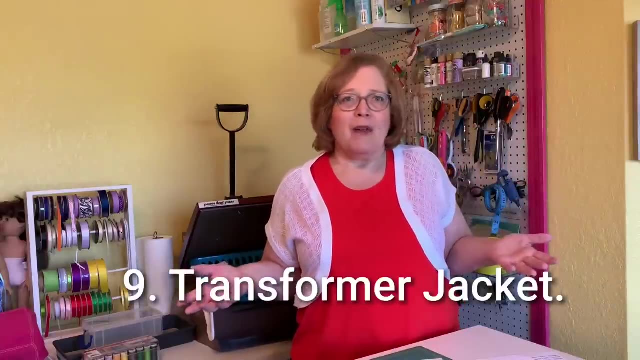 So then you turn it into a backpack and you carry it on your back while you need it, and then when you're in the airplane, it's a pillow. So, because it's nice and soft too, So you could use it as a pillow. and then, when you get to where you're going, if it's cooler than it was where you, 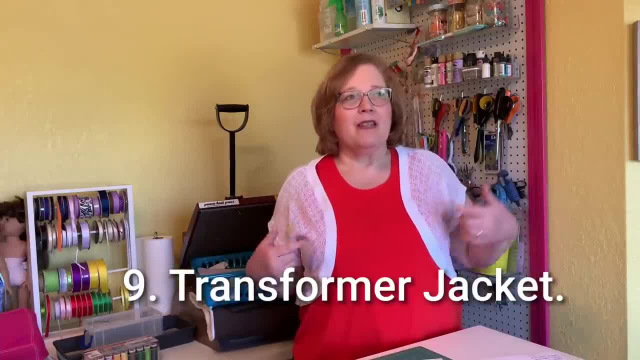 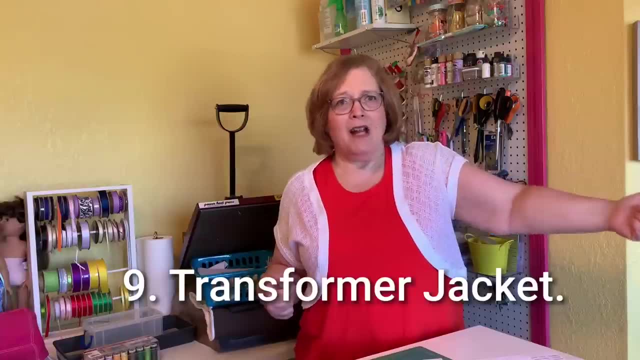 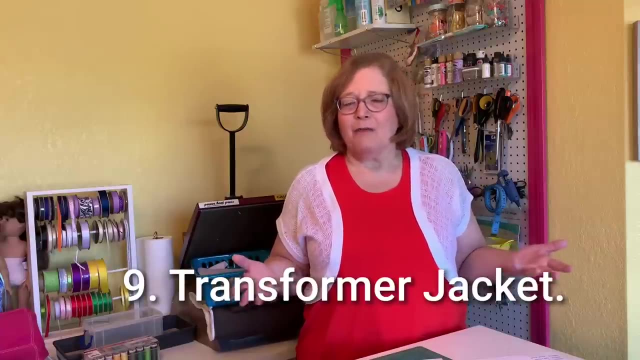 left you can throw it on. Or, for instance, when we come back from Mexico. it's March and it's usually still pretty cold here, but we're leaving 85-90 degrees and coming back to winter pretty much. So having that jacket would be really nice, because I don't carry a heavy coat with me. 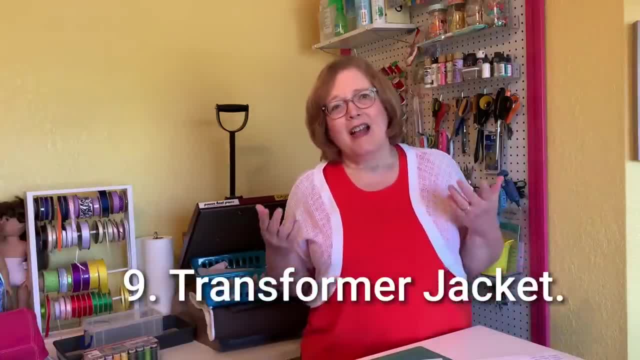 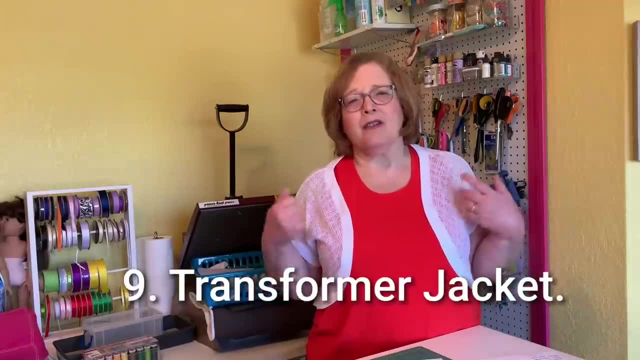 I just freeze until I get to the car, So I usually try to have a hoodie with me. but this way it doesn't have to count really as a carry-on or anything. You can just throw it on your back and and it doubles as a pillow. 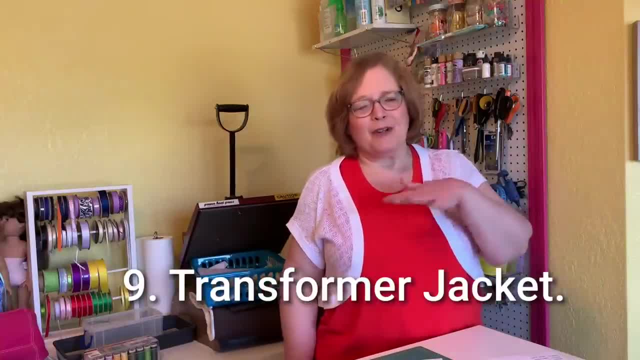 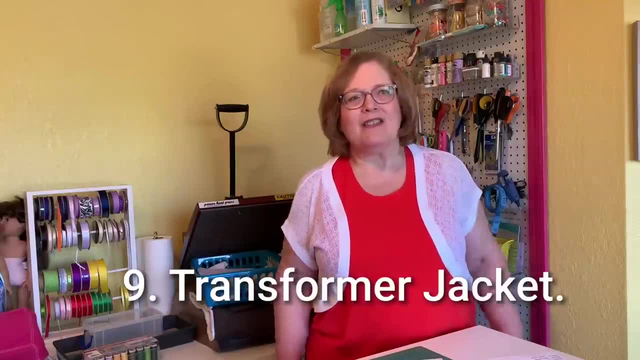 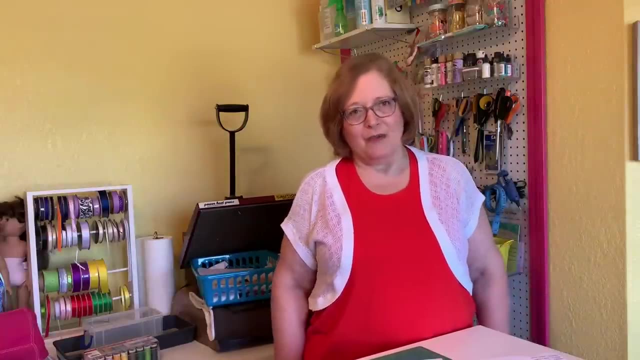 So I think it would be really great for airline travel for adults, but that's not what this video is about. But it's a just got endless possibilities and I think kids just love those kind of things. Now, number 10 is doll clothes. 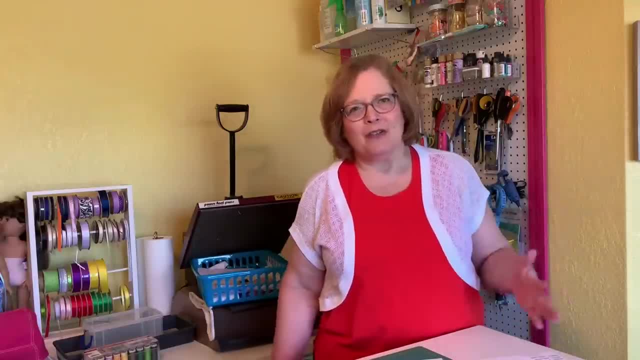 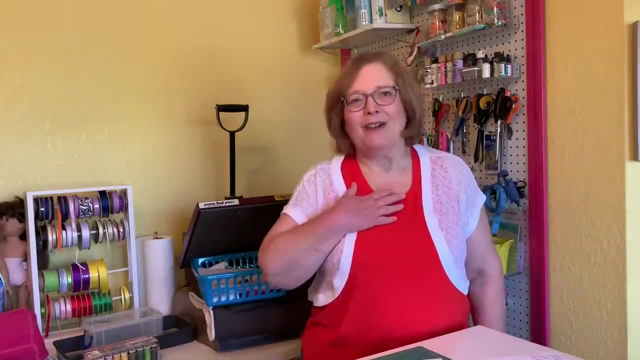 So anytime you can make American Girl doll clothes for a little girl if they're into that, it just they're so thrilled And I love doll clothes too, so I tend to make a lot of them. I've done everything from cheerleader outfits for Ohio State to princess dolls. 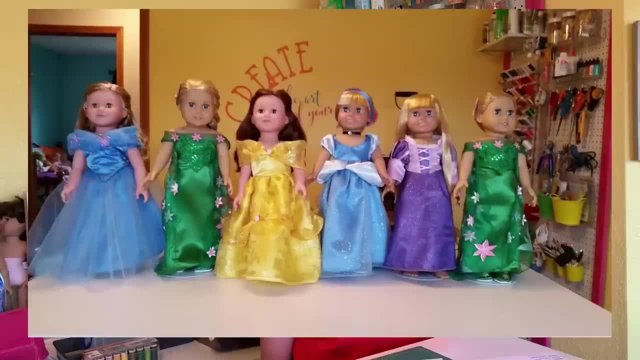 Now, princess dolls would be my number one tip when it comes to dolls. So you go to Michaels and you buy the dolls with your 40% coupon. They end up being between 10 and 15 dollars. You come home, you style hair the way for a Disney princess. 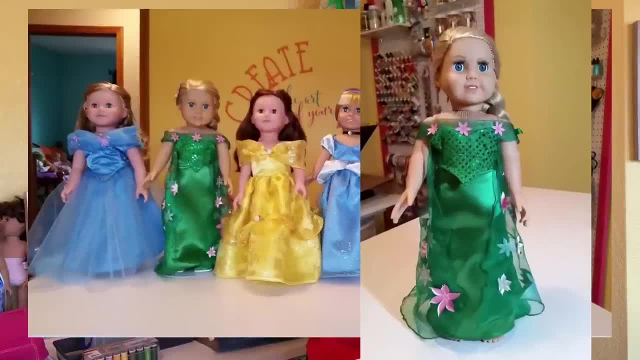 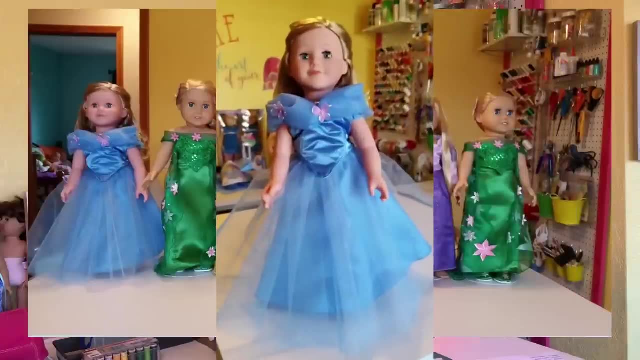 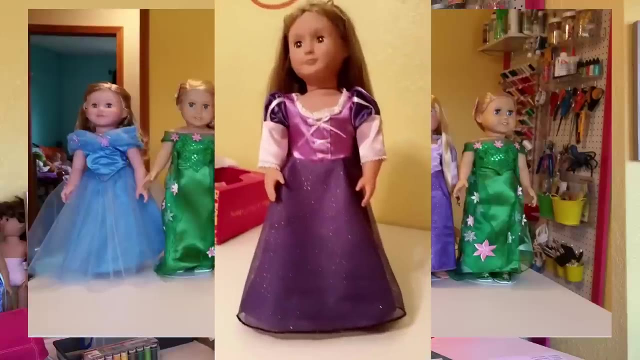 and then you go ahead and you make the gown of whatever the princess is, and you go ahead and make the Disney princess- And I'll show you a picture here of several that I did one Christmas And they're just thrilled with them and they cost a fraction of what they cost at the Disney Store And 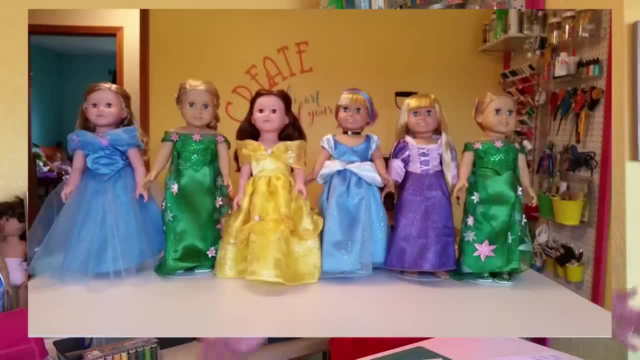 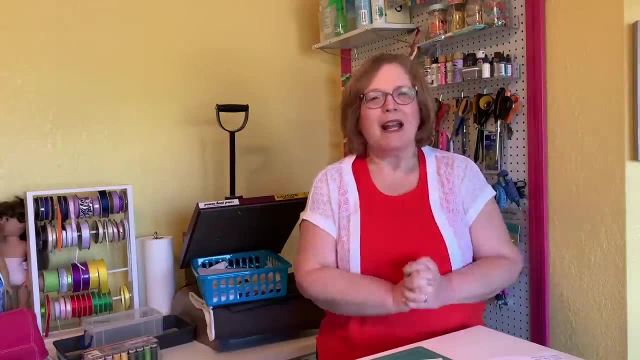 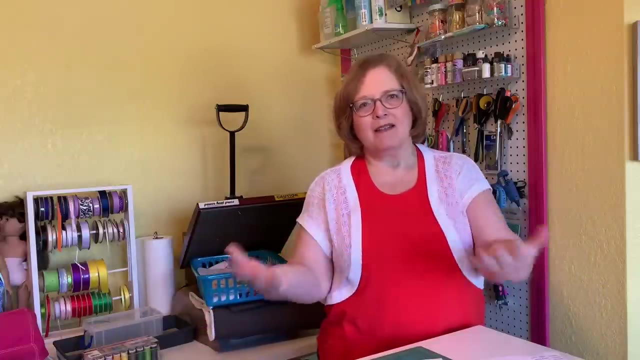 Grammy made them, So All right. so that is my top 10 things for to sew for kids, and I have one bonus thing: Why not sew with them? It's just so fun, They love it and you could be teaching them, passing your skill down to the next. 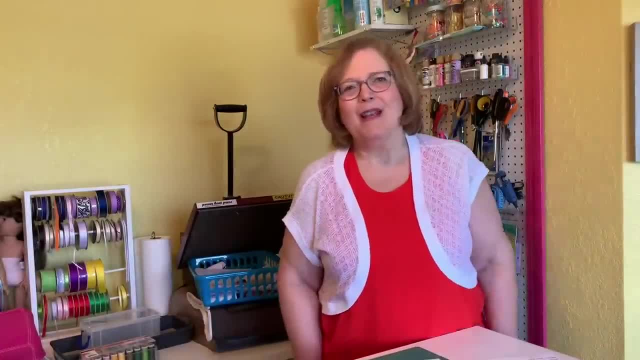 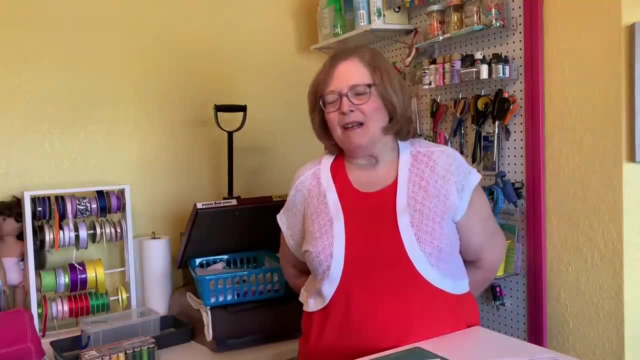 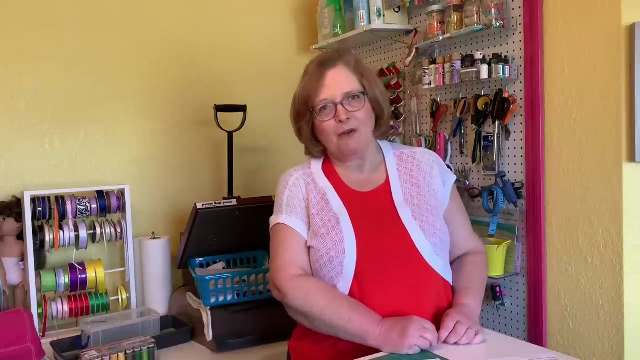 generation. Whether they be grandkids, kids, nieces, nephews, whatever, Everybody has kids in their life to sew for All right. so a lot of you have asked me how you can support the channel. Some have asked me: do I have a Ko-Fi account? 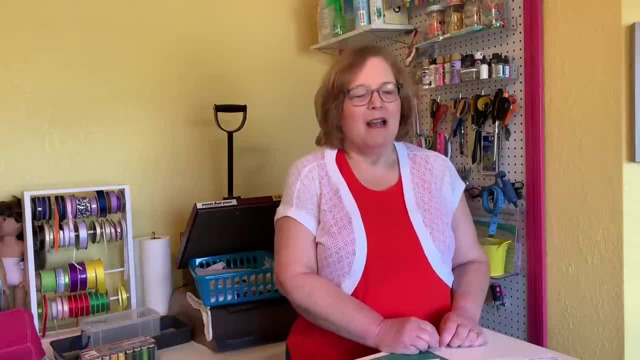 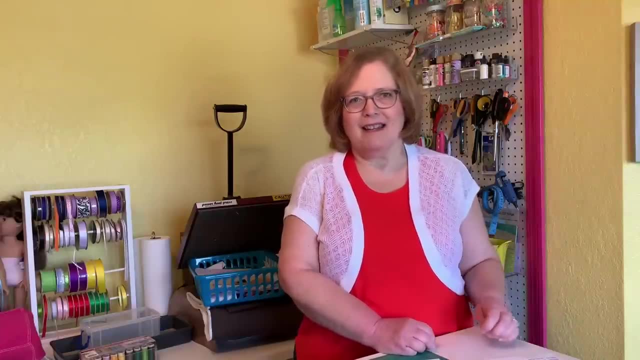 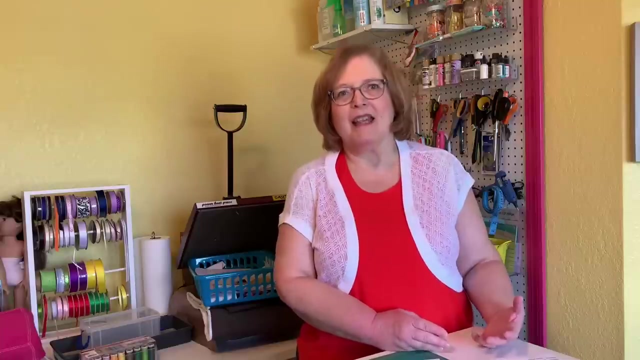 And just different ways that they can say thank you. I'm just not really It's not really my nature to like solicit that stuff, but the channel does cost money to produce. So I will share with you just a few ways that you can support this channel and just leave it at that, okay. 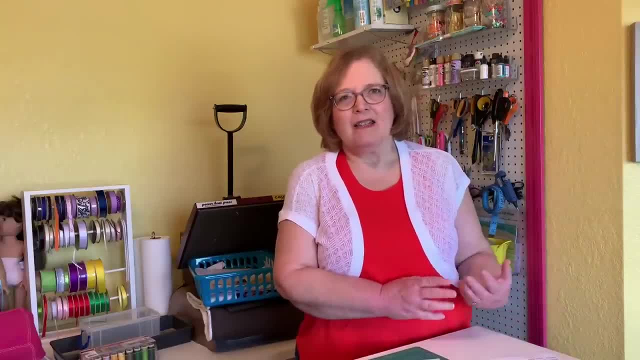 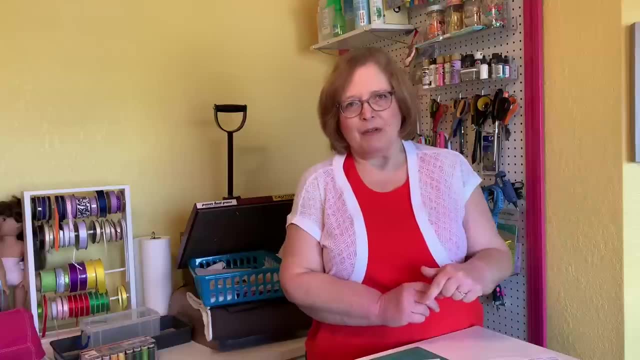 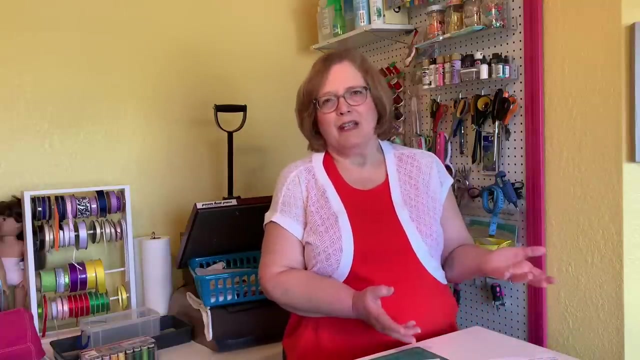 I do have a Ko-Fi account. It is Dorothy's Daughter Sews, and I will put the link to the Ko-Fi account down in the description. That is one way you can help Another Ko-Fi if you're not familiar with it. it's kind of a tip jar for creators. 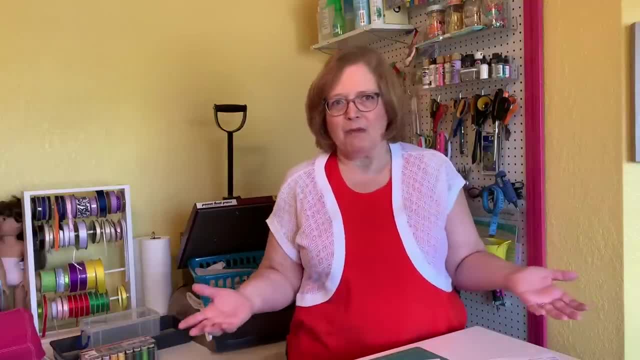 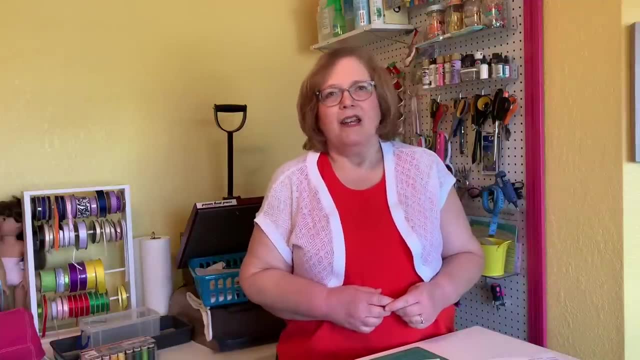 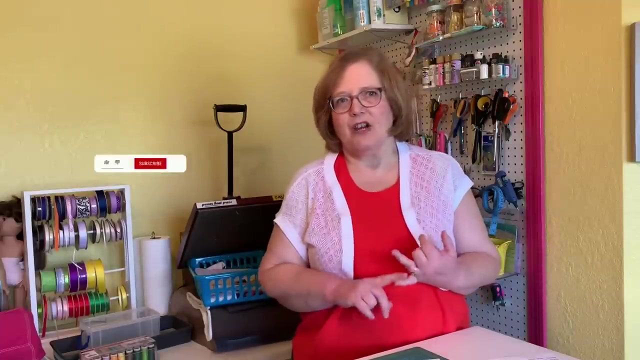 So if somebody does a YouTube video that blesses you and they have a Ko-Fi account, you can go ahead and contribute. It's just a kind of a way to say thank you, Another way that you can really support this channel. the simplest thing that doesn't cost any money is to like, share and subscribe. 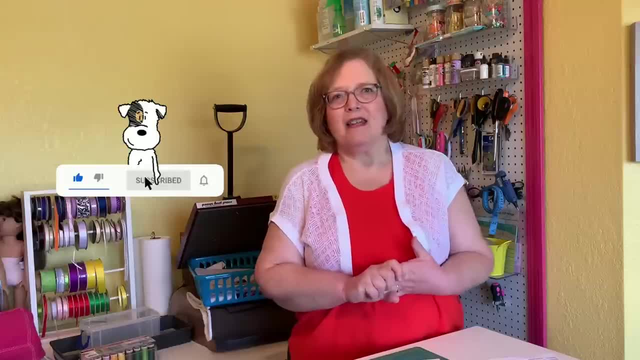 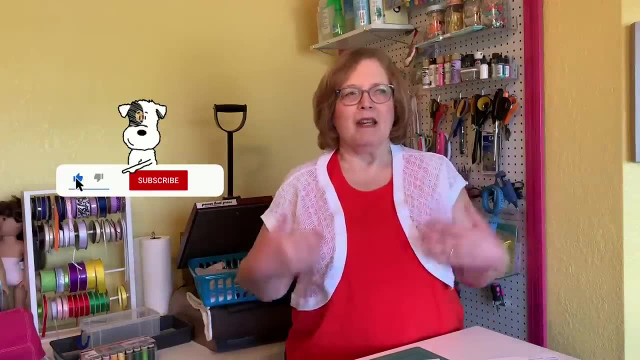 to the channel. Those all help YouTube to see that any way that YouTube sees this channel as one that people want to watch gets the channel out more, which means that the resources then come back to do even better videos and more videos. 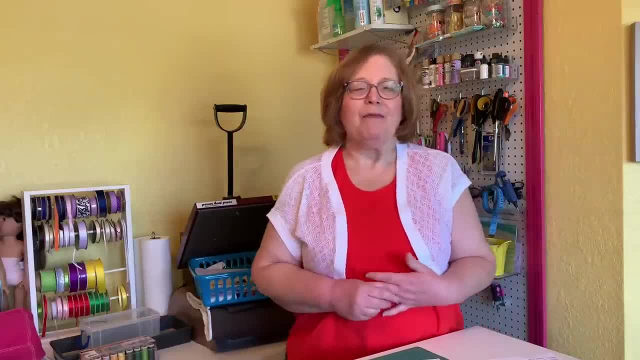 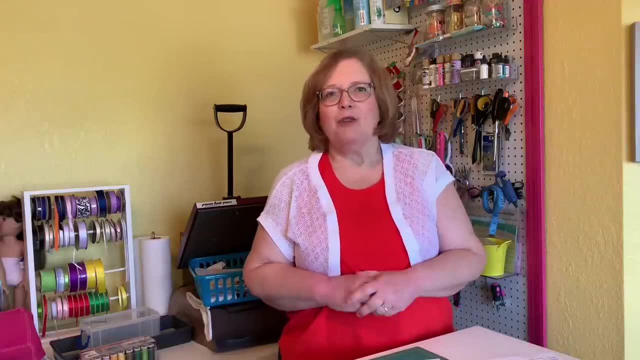 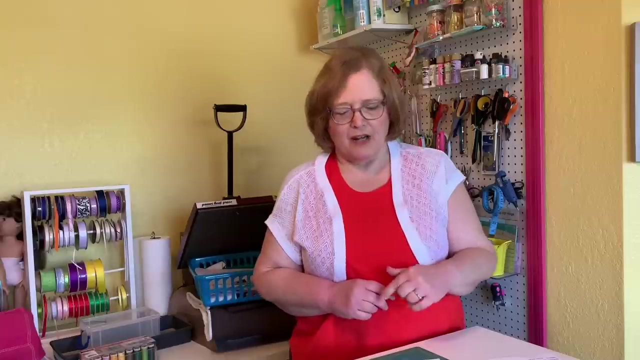 So that is the simplest way to support this channel. Another way is I have an Amazon storefront and I always link that in my description box. Anything you go to Amazon for if you go to that link first, it'll get credited back to this channel. 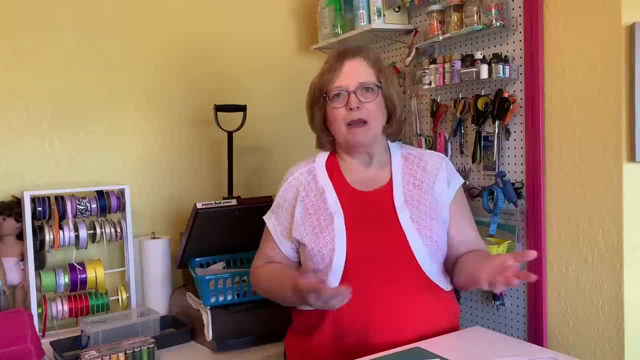 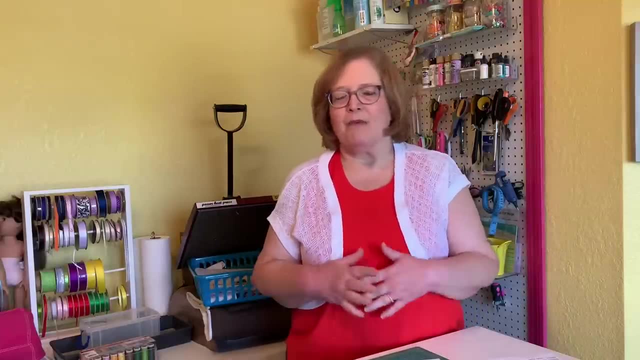 And another thing is just to follow the affiliate links to the various pattern designers and whatnot. Those all add up too. So those are some ways that you can help this channel And I- you know I don't want to really like make a huge deal about it. 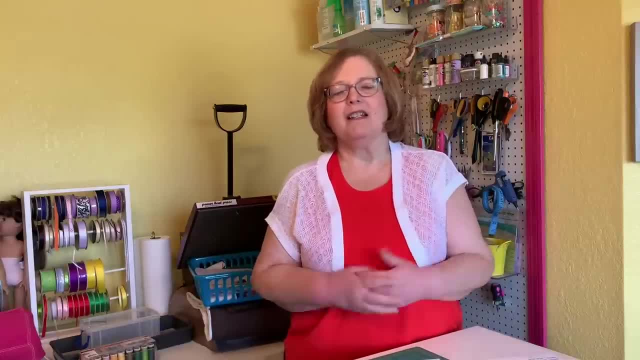 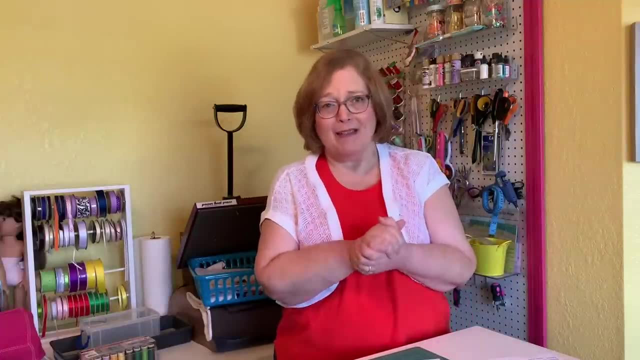 but I just wanted to put that out there. If you would like to help, that is one way you can do that. Well, I hope you have a fantastic weekend. I'm going to be spending it with four of my littles, and 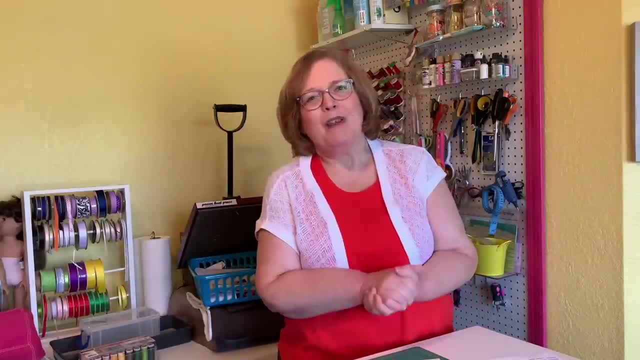 I'm just looking forward to it very much, So I hope that you have a fantastic weekend. Have a great day and happy sewing. Thanks for watching.